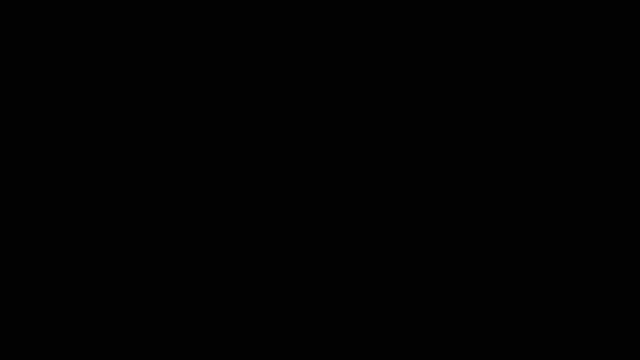 In this video, we're going to talk about how to graph polynomial functions using things such as n-behavior, multiplicity and even finding the zeros, So let's begin by taking down some notes. first, Let's begin our discussion with a graph of: y equals positive, x squared. 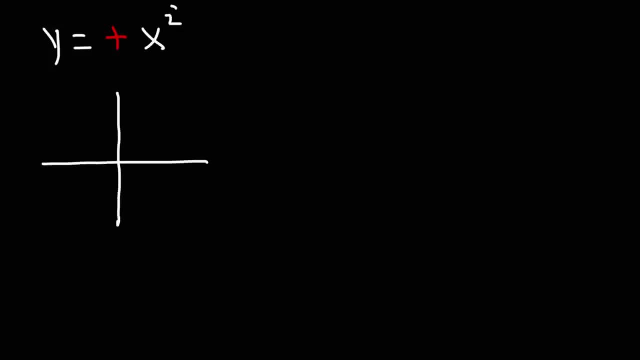 So this is an even function with a degree of 2.. Even functions are symmetrical about the y-axis, And so this is the shape of the y equals x squared graph: The n-behavior towards the left is up and the n-behavior towards the right is up. 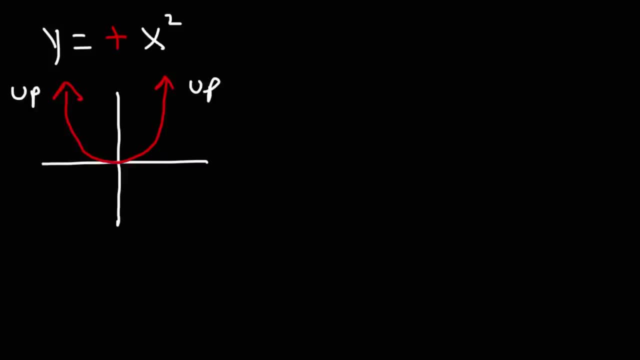 Now there's other ways in which you can describe the n-behavior of this graph. On the right side, as x approaches positive infinity, y approaches positive infinity. So here's how you can visualize it: As you move towards the right along the x-axis, as you go towards positive infinity. 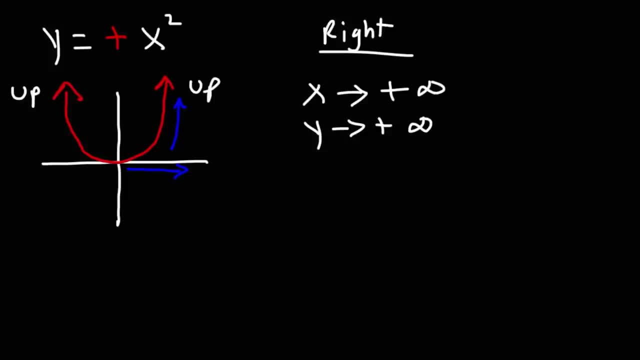 the values along the y-axis are increasing. You're going up towards positive infinity on the y-axis. Now the n-behavior for this graph on the left: as x approaches negative infinity, y approaches positive infinity. So you can visualize this graph: as x approaches negative infinity, y approaches positive infinity. 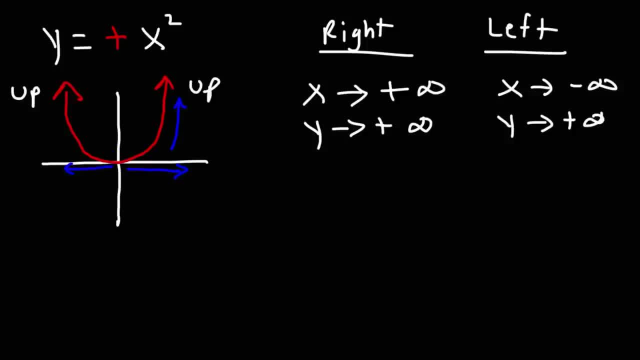 As we go to the left, we can see the y-values are increasing. So this is another way in which you can describe the n-behavior of that graph. Now let's consider another example. In this case it's going to be: y equals negative, x squared. 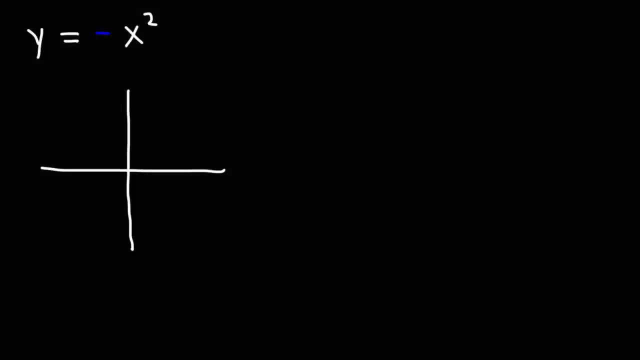 Now, this is also an even function, so we're going to have symmetry along the y-axis, But we have a negative sign. The leading coefficient is negative, So this is going to reflect over the x-axis. So the graph is going to look like this: 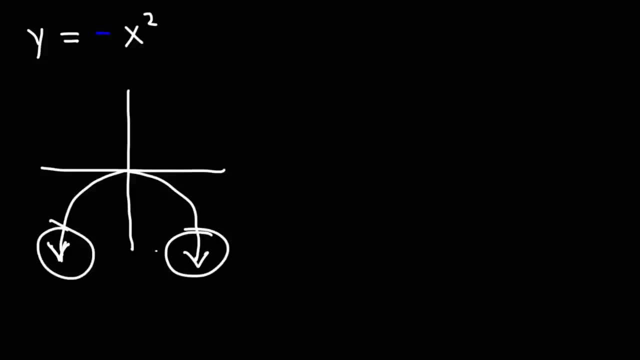 As we can see, the n-behavior on the left is down and it's also down on the right, But we can express it this way just like before. So on the left side, as x approaches positive infinity, that is, as we go towards the right. 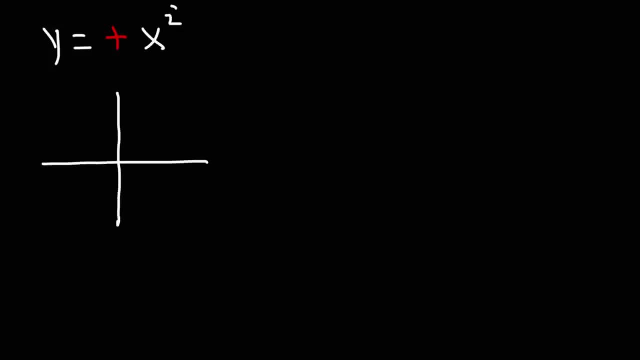 So this is an even function with a degree of 2.. Even functions are symmetrical about the y-axis, And so this is the shape of the y equals x squared graph: The n-behavior towards the left is up and the n-behavior towards the right is up. 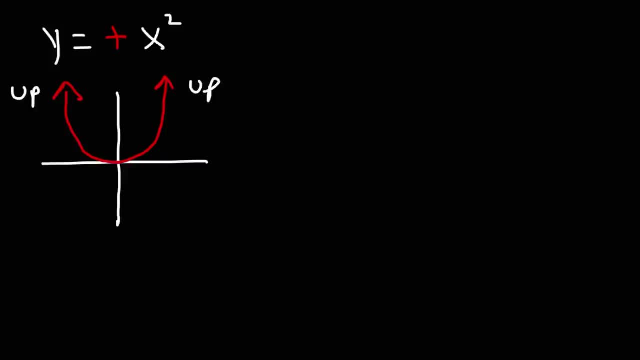 Now there's other ways in which you can describe the n-behavior of this graph. On the right side, as x approaches positive infinity, y approaches positive infinity. So here's how you can visualize it: As you move towards the right along the x-axis, as you go towards positive infinity. 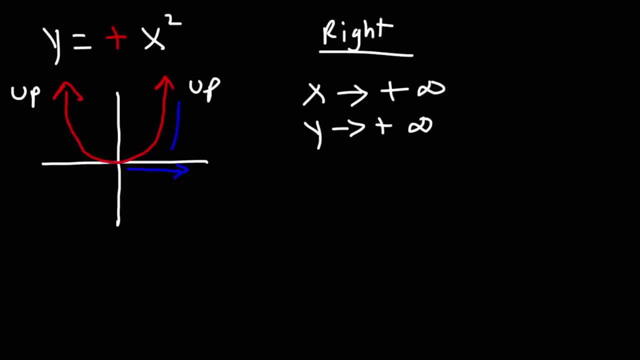 the values along the y-axis are increasing. You're going up towards positive infinity on the y-axis. Now the n-behavior for this graph on the left: as x approaches negative infinity, y approaches positive infinity. As we go to the left we can see the y-values are increasing. 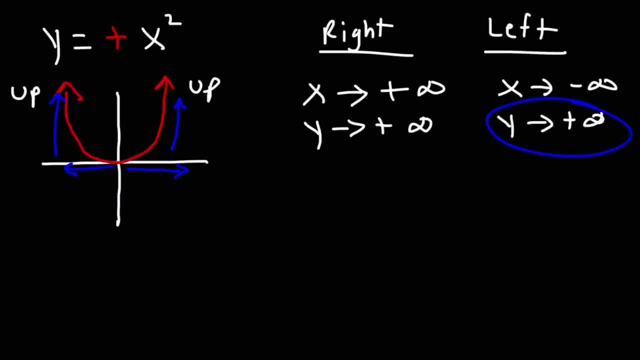 So this is another way in which you can describe the n-behavior of that graph. Now let's consider another example. In this case it's going to be y equals negative x squared. Now this is also an even function, so we're going to have symmetry along the y-axis. 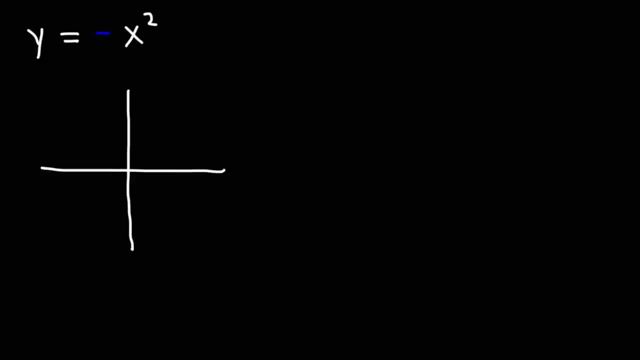 But we have a negative sign. The leading coefficient is negative, So this is going to reflect over the x-axis. So the graph is going to look like this: As we can see, the n-behavior on the left is down and it's also down on the right. 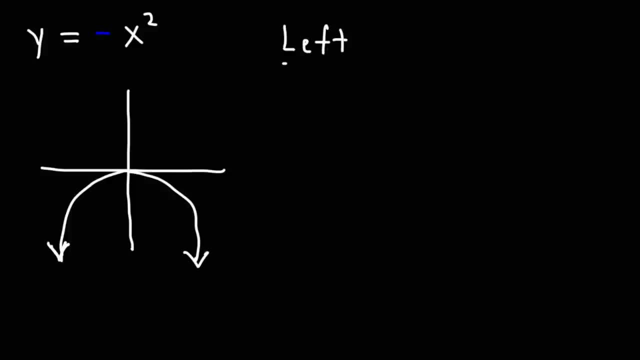 But we can express it this way, just like before. So, on the left side, as x approaches positive infinity, that is, as we go towards the right, what happens to the y-value? Well, We can see that. We can see that the y-value is decreasing. 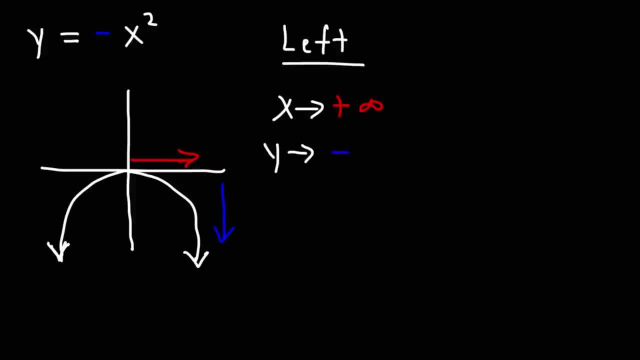 It's becoming more negative, so it's approaching negative infinity. So that's the n-behavior I put left. This should be on the right side, Because x is going towards positive infinity. So that's the n-behavior towards the right side. 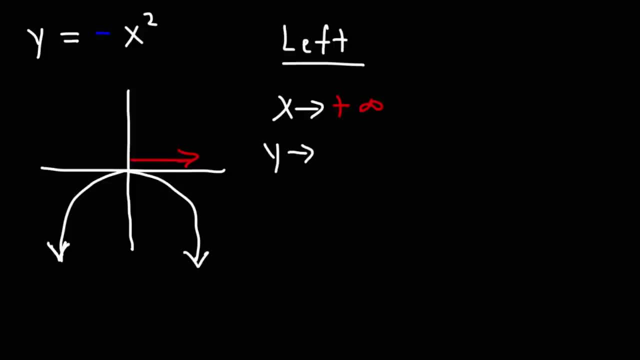 what happens to the y-value? Well, we can see that x approaches positive infinity. That is as we go towards the right. what happens to the y-value? Well, we can see that the y-value is decreasing. It's becoming more negative, so it's approaching negative infinity. 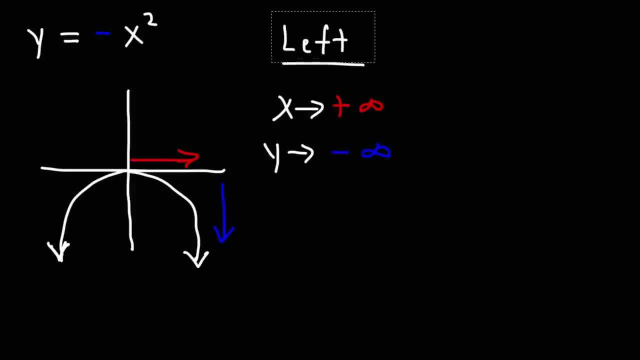 So that's the n-behavior I put left. This should be on the right side, because x is going towards positive infinity. So that's the n-behavior towards the right side. Now towards the left side, that is when x goes to negative infinity. 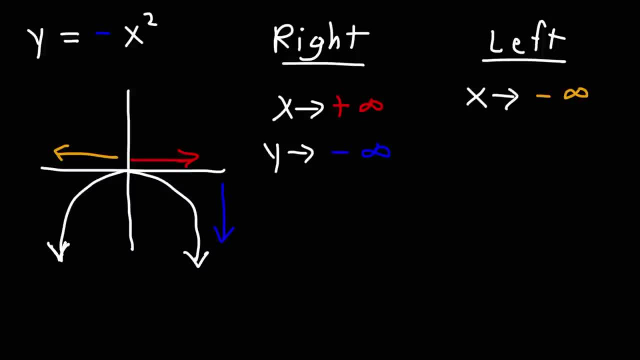 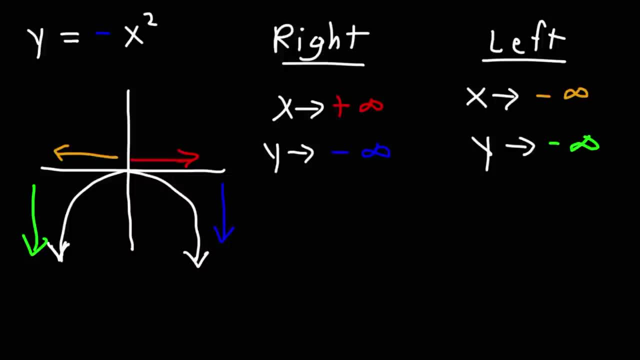 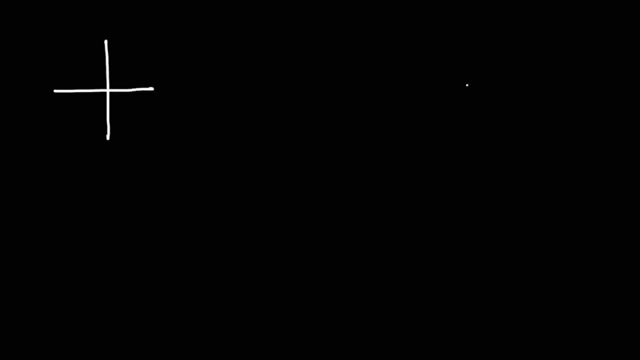 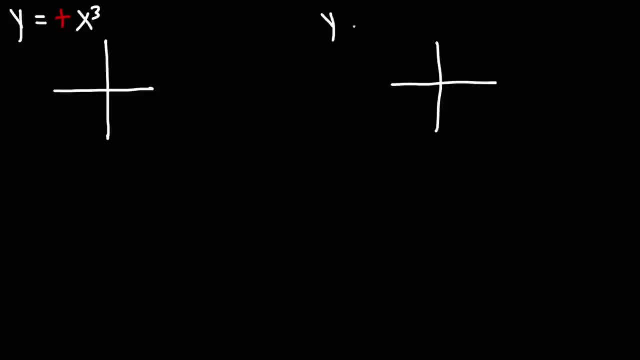 Notice what's happening. and y equals negative x cubed, And I'll give you the shape of these graphs. So positive x cubed looks like this: It starts from the bottom and then- let me draw this better- It curves towards zero. 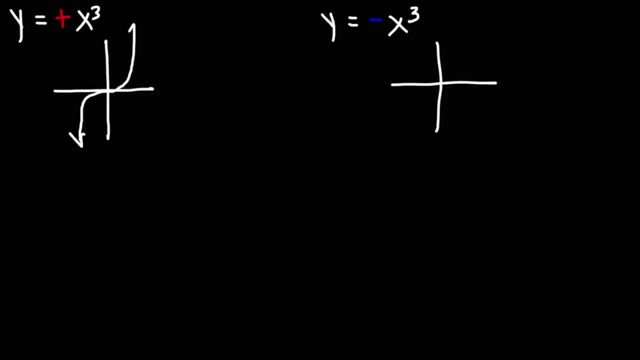 It's actually almost horizontal at the origin and then it goes back up. So right here you have like a horizontal tangent. Now for y equals negative x squared. it reflects about the origin. So it looks like that And we still have that same horizontal tangent where it touches the x-axis. 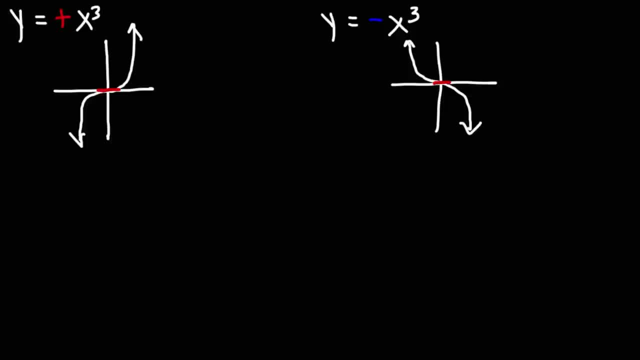 So go ahead and describe the left and the right end behavior for these two graphs. So let's start with the left side. As x approaches negative infinity, what happens to y? Well, as we go towards the left, we can see that the y values are becoming more negative. 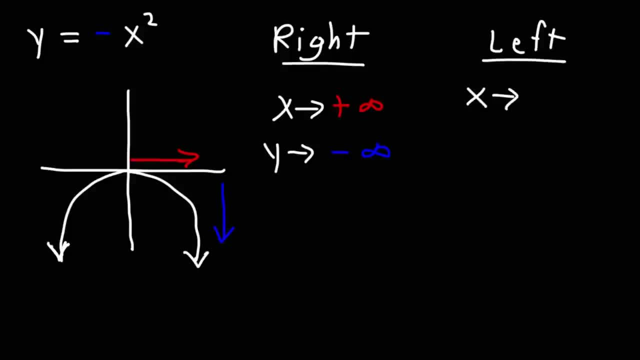 Now towards the left side, that is when x goes to negative infinity. So we're going towards the left. Notice what's happening to the y-value, The y-values. they're also becoming more negative. So y is approaching negative infinity. So that's one way in which you could describe the n-behavior of a particular graph. 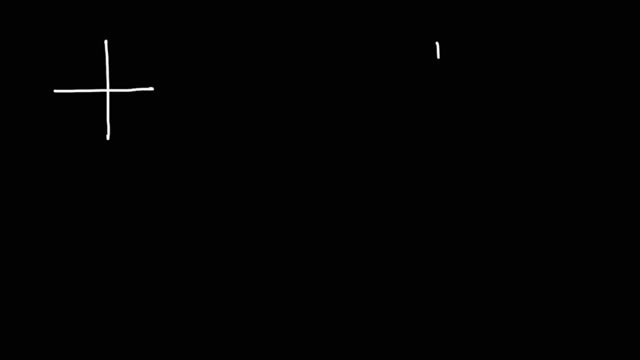 Now, for the sake of practice, go ahead and describe the n-behavior for these two graphs: y equals positive, x-cubed, x-cubed, x-cubed, x-cubed, And y equals negative- x-cubed. 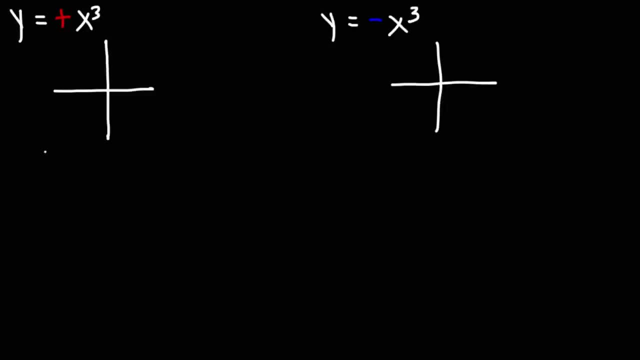 And I'll give you the shape of these graphs. So positive x-cubed looks like this: It starts from the bottom And then- let me draw this better- It curves towards zero. It's actually almost horizontal at the origin, And then it goes back up. 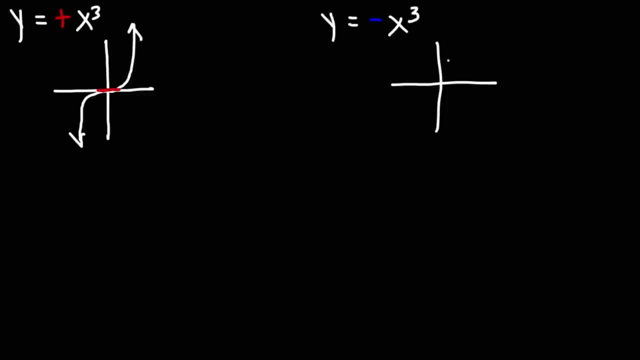 So right here you have like a horizontal tangent. Now for y equals negative x-squared, It goes up, It reflects about the origin, So it looks like that, And we still have that same horizontal tangent where it touches the x-axis. 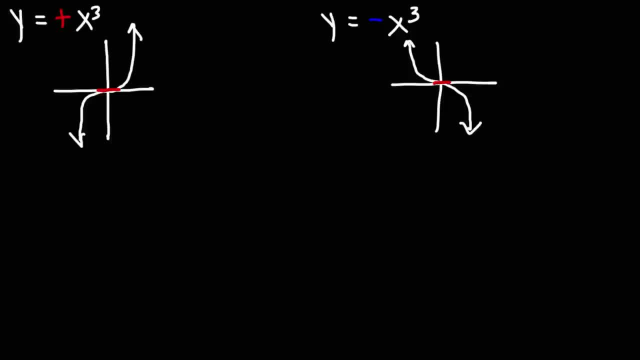 So go ahead and describe the left and the right n-behavior for these two graphs. So let's start with the left side. As x approaches negative infinity, what happens to y? Well, As we go towards the left, we can see that the y-values are becoming more negative. 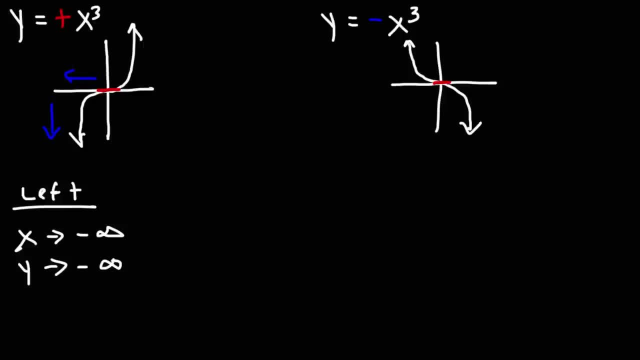 Y approaches negative infinity. Now for the right side. as x goes to positive infinity, y goes up. It goes towards positive infinity as well. So that's the n-behavior for positive x-cubed. Now let's look at the right side. 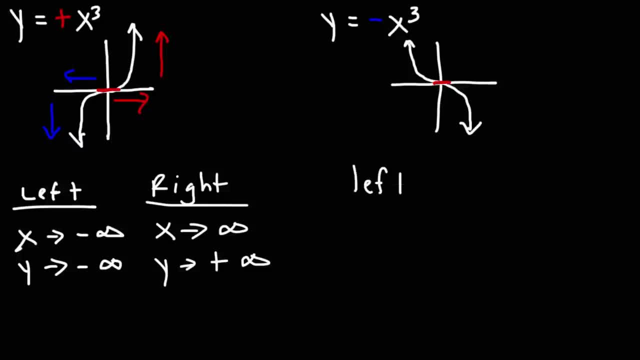 Let's look at the left side Now. let's do the same for negative x-cubed. As x approaches negative infinity, what happens to y? As we go towards the left, the y-values are increasing in the positive y-direction, So it goes towards positive infinity. 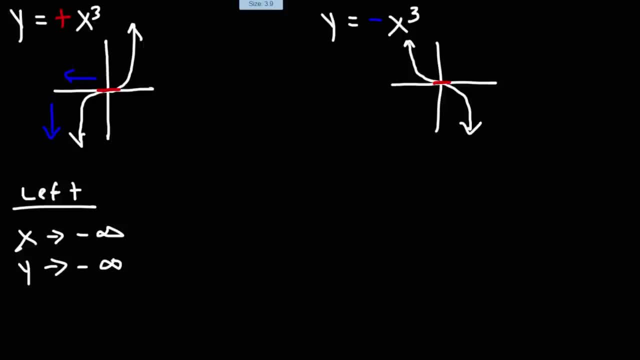 y approaches negative infinity. Now for the right side: as x goes to positive infinity, y goes up, It goes towards positive infinity as well. So that's the end behavior for positive x cubed. Now let's do the same for negative x cubed. 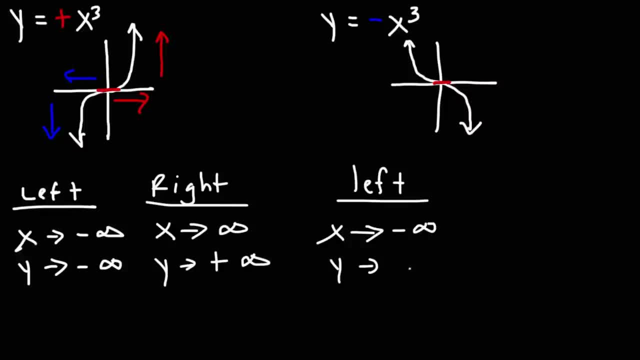 As x approaches negative infinity. what happens to y? As we go towards the left, the y values are increasing in the positive y direction. So it goes towards positive infinity. It's going up And for the right end behavior as x approaches positive infinity. 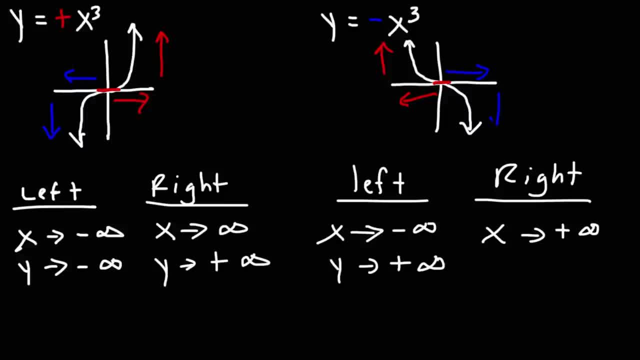 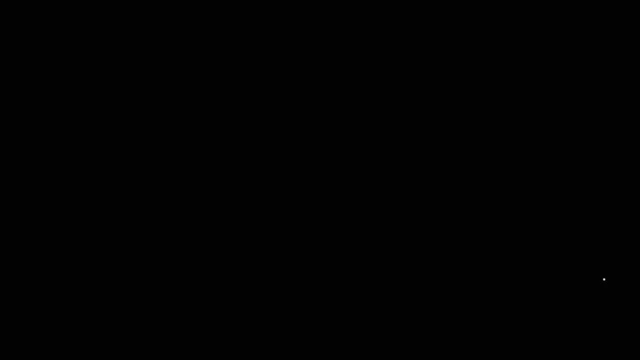 as we move towards the right side, we can see that the curve is going down. So y approaches negative infinity. So now let's put everything together. Let's start with the even functions. So y equals positive x squared. What you need to know is that the end behavior is: 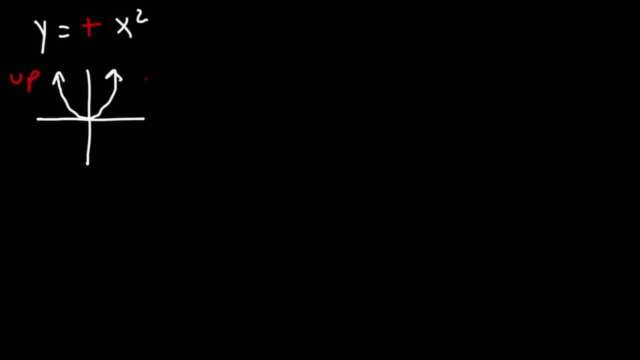 up up Now. the same is true for y is equal to positive, x to the fourth. This graph looks similar. The end behavior is up on the left and up on the right. So anytime you have a polynomial with an even degree and a positive leading coefficient, 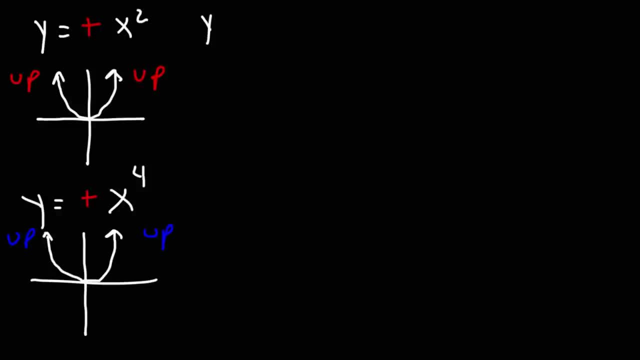 the end behavior will be up up. Now, if we have negative x squared, that does not look like a 2, let's do that again. The end behavior is going to be down on the left and down on the right, So I'm just going to use d to represent down. 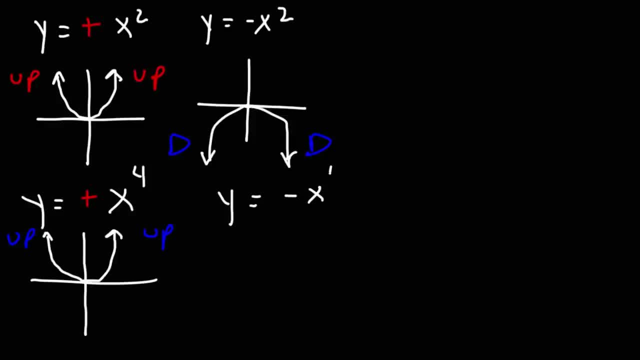 Now for y equals negative x to the fourth, the situation is similar. It's going to be down on the left and down on the right as well. So anytime you have a polynomial with an even degree or an even exponent, it's either up up or down down. 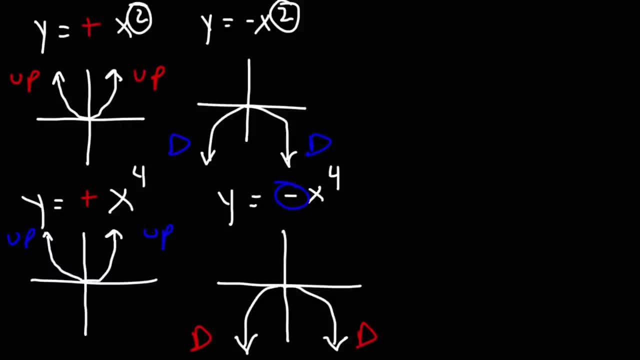 The difference is based on the sign of the leading coefficient. If it's negative, it's down down, But if the leading coefficient is positive, it's going to be up up. Now let's consider the examples where the exponent is odd. 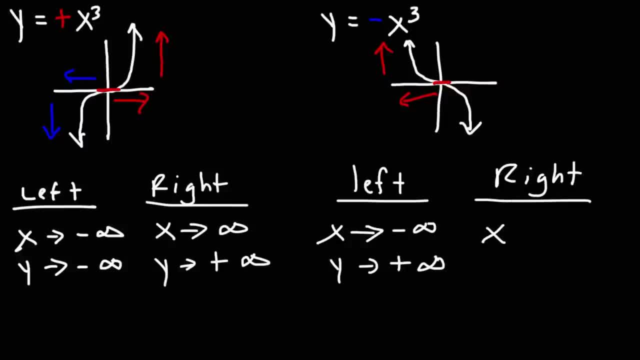 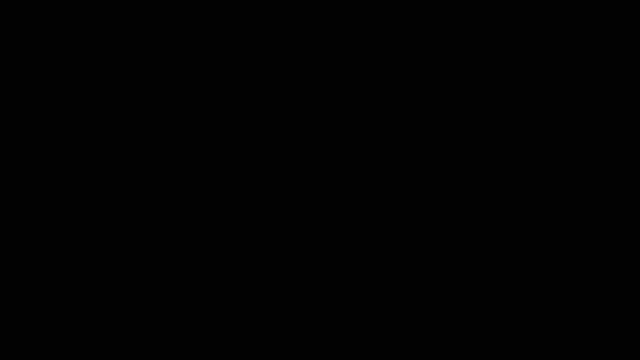 It's going up And for the right n-behavior, as x approaches positive infinity. as we move towards the right side, we can see that the curve is going down, So y approaches negative infinity. So now let's put everything together. 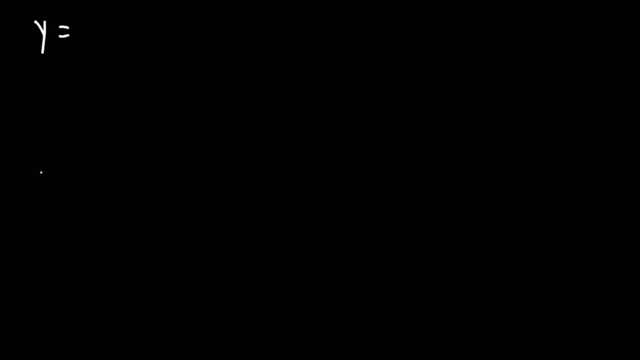 Let's start with the even functions. So y equals positive x-squared. What you need to know is that the n-behavior is up up Now. the same is true for y is equal to positive x-squared, x to the fourth. 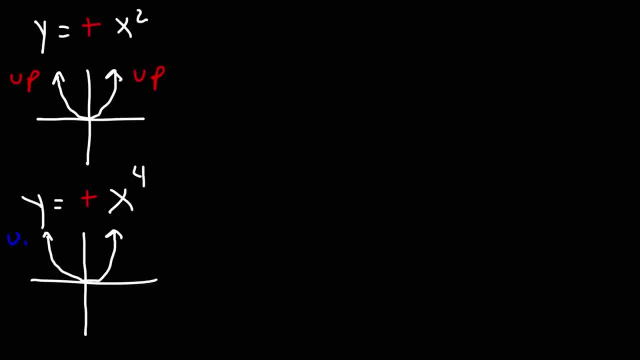 This graph looks similar. The n-behavior is up on the left and up on the right. So any time you have a polynomial with an even degree and a positive leading coefficient, the n-behavior will be up up. Now, if we have negative x-squared, that does not look like a 2.. 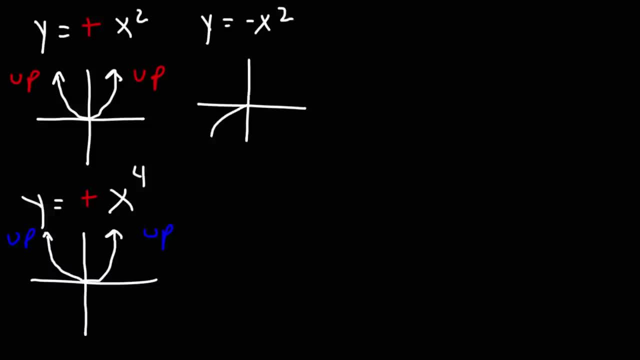 Let's do that again. The n-behavior is going to be down on the left and down on the right, So I'm just going to use d to represent down Now, for y equals negative x. to the fourth, the situation is similar. 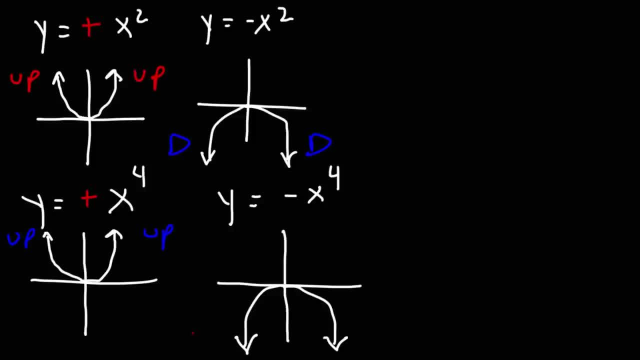 It's going to be down on the left and down on the right as well. So any time you have an even exponent, Either up, up or down down. The difference is based on the sign of the leading coefficient. If it's negative, it's down down. 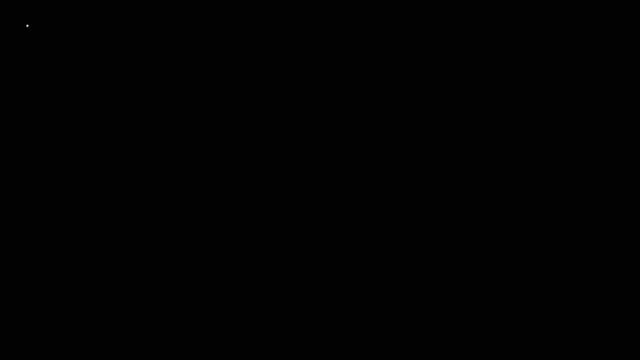 But if the leading coefficient is positive, it's going to be up up. Now let's consider the examples where the exponent is odd. So, going back to positive x-cubed, The n-behavior is down on the left, Up on the right. 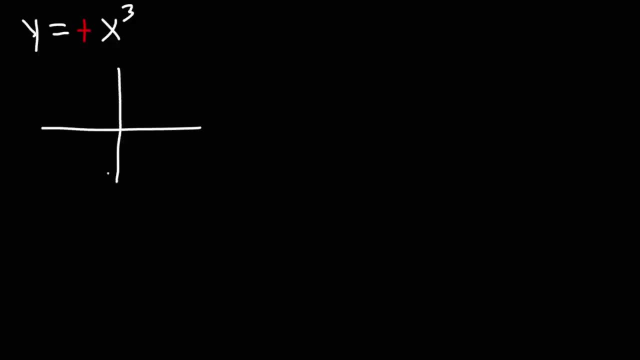 So, going back to positive x cubed, the end behavior is positive x cubed Down on the left, up on the right. Now this is similar to y is equal to positive x to the first power. But this is going to be a straight line. 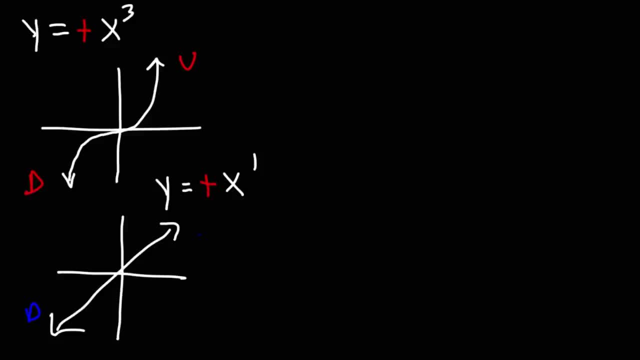 But the end behavior is still the same. It's down on the left, up on the right. So anytime the exponent is odd, the end behavior is going to alternate. It's going to be either down, up or up down If the leading coefficient is positive. 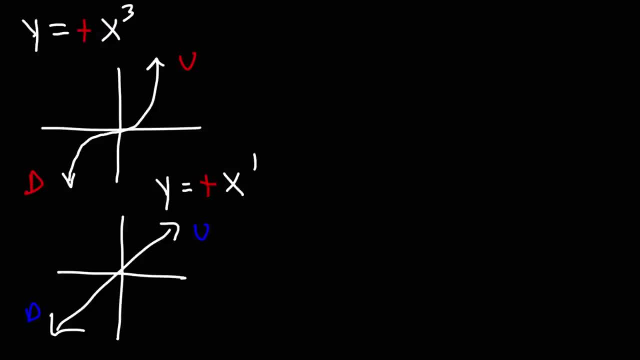 it's going to go from down to up, So it's going to be increasing. Now, if the leading coefficient is negative, we're going to get the reverse situation. So instead of going from down up, it's now going to be up. 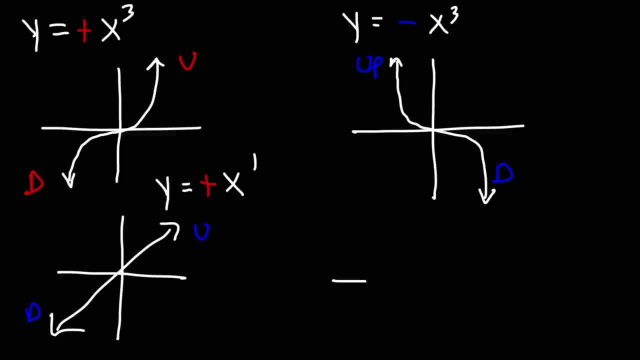 and then it's going to go down, And the same is true for y equals negative x to the first power. It's a straight line, but it's going to go in this direction. It's initially up on the left, but it's going to be down on the right. 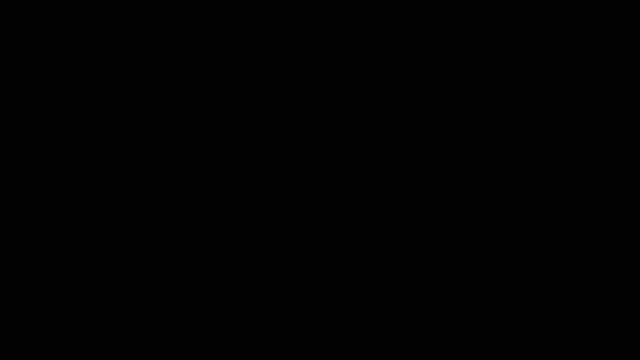 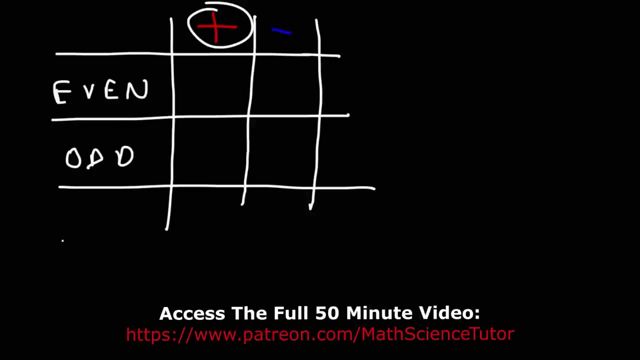 So now let's summarize this in a table. You may want to write this down. So when the exponent or the overall degree of the polynomial function is even, and if the leading coefficient is positive, the end behavior will be up up If we have a degree that's even. 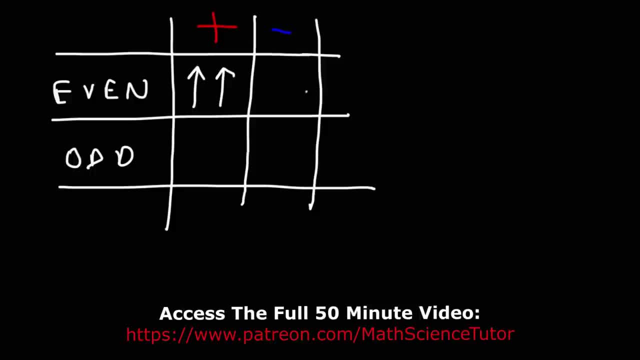 but the leading coefficient is negative, then it's going to be down, down. That's the end behavior. Now, if we have an odd degree with a positive leading coefficient, it's going to be down at first and then it's going to be up. 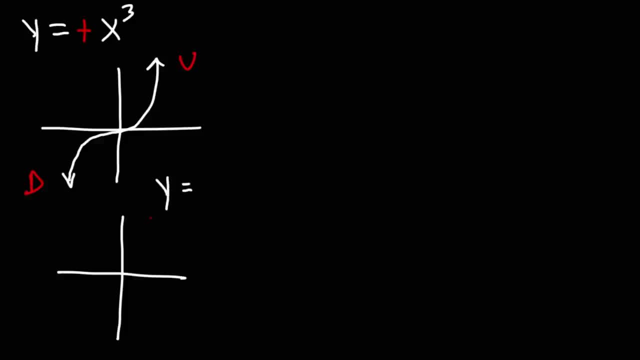 Now this is similar to y is equal to positive x to the first power. But this is going to be a straight line. But the n-behavior is still the same. It's down on the left, up on the right, So any time the exponent is odd, the n-behavior is going to alternate. 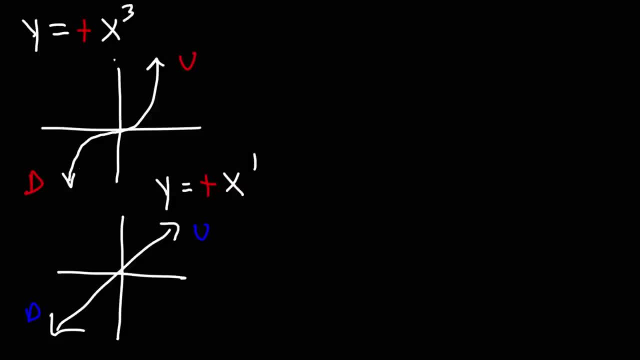 It's going to be either down up or up down. If the leading coefficient is positive, It's going to go from down to up, So it's going to be increasing. Now, if the leading coefficient is negative, we're going to get the reverse situation. 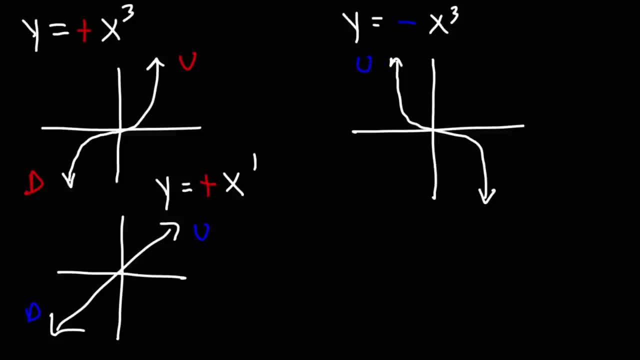 So, instead of going from down up, it's now going to be up and then it's going to go down. And the same is true for y equals negative x to the first power. It's a straight line. It's a straight line, but it's going to go in this direction. 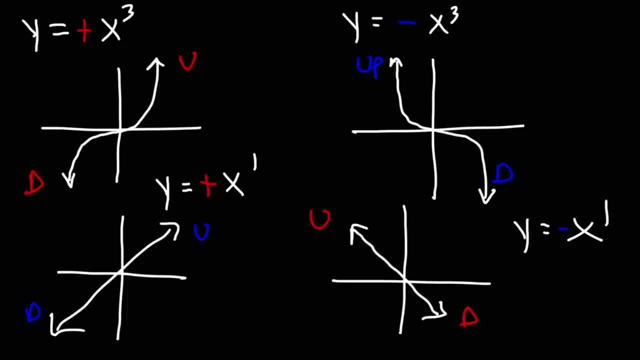 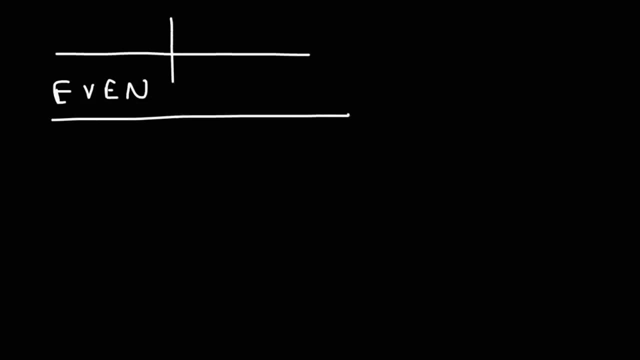 It's initially up on the left, but it's going to be down on the right, So now let's summarize this in a table. You may want to write this down. So, when the exponent or the overall degree of the polynomial function is even, and if 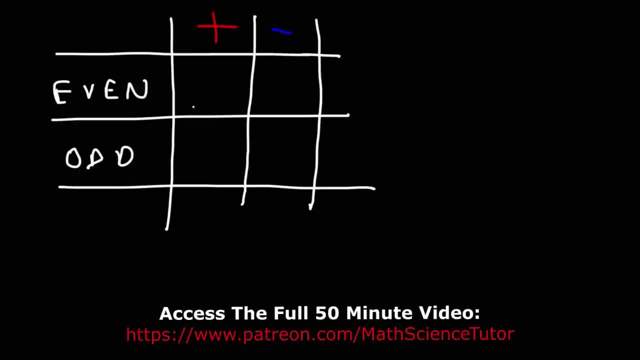 the leading coefficient is positive, the n-behavior will be up up. If we have a degree that's even, but the leading coefficient is negative, the n-behavior will be up up. If the leading coefficient is negative, then it's going to be down, down. 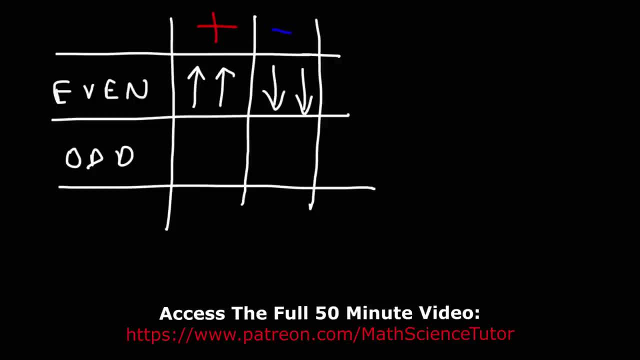 That's the n-behavior. Now. if we have an odd degree with a positive leading coefficient, it's going to be down at first and then it's going to be up. If it's odd and negative, it's going to be up and then down. 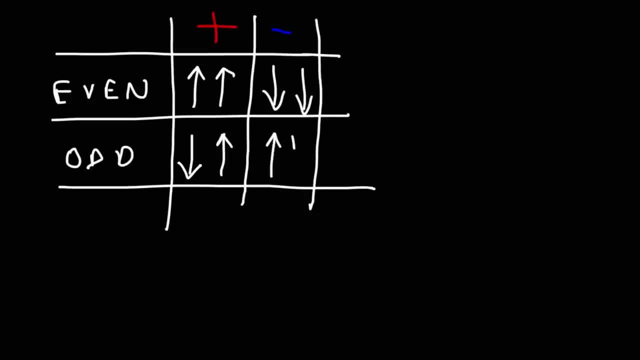 If it's odd and negative, it's going to be up and then down. Now let's talk about the behavior of the graph near an x-intercept. I'm going to explain this more later in this video, but I'm going to explain it. 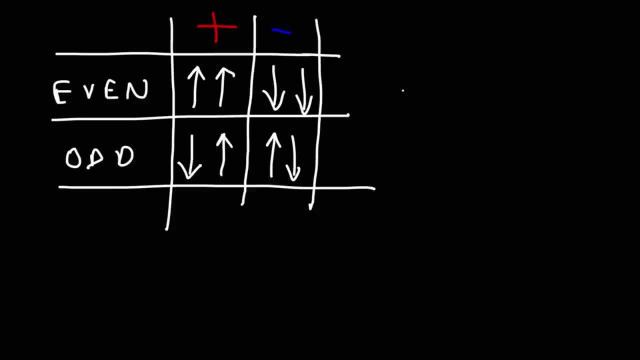 but for now you want to write this down. So let's say, the multiplicity of a particular x-intercept or a particular zero is one. This is going to look like the graph: y equals x to the first power. So at that, zero. 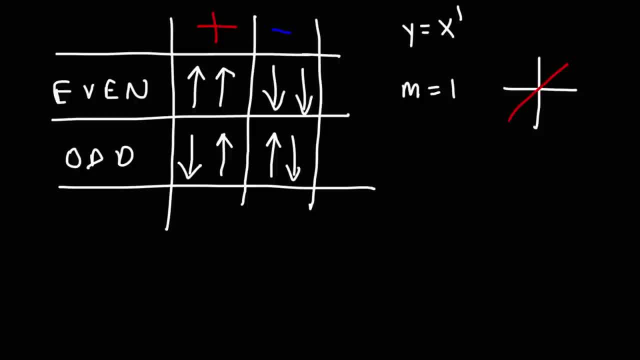 it's simply just going to cross the x-axis, basically in a straight line. Now, the angle of the straight line can vary, so you don't have to be too specific about that. If the angle of the straight line is 1,. if the multiplicity is 2,. 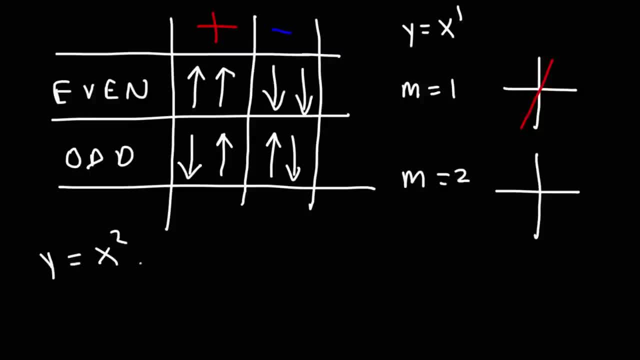 it's going to look like the graph y equals x squared. It's not going to cross the x-axis but it's going to touch or bounce on the x-axis, much in a similar way to the graph y equals x squared If the multiplicity is 3 for a particular zero or x-intercept. 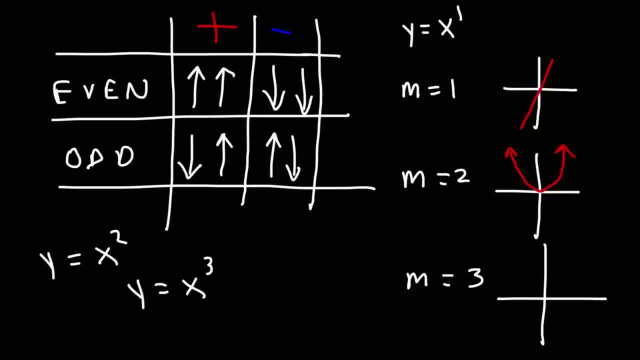 it's going to look similar to x cubed, but at that x-intercept. So if you think of the graph of x cubed, it looks something like this. So you're going to have that same shape here, but you're going to have 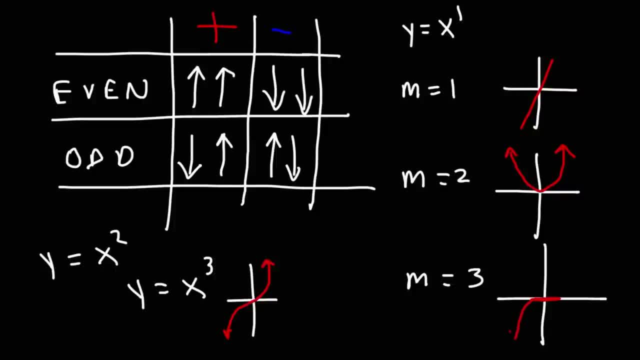 the behavior at that zero is going to be horizontal. So make sure you understand that if the multiplicity is 1, the behavior at the x-intercept is going to be like a straight line. It's going to cross the x-axis in a straight line. 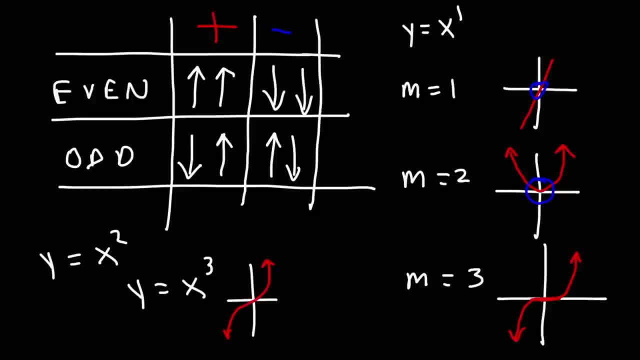 If the multiplicity is 2, at that x-intercept it's not going to cross the x-axis, but it's going to bounce. it's going to bounce on, you know that point. And then if the multiplicity is 3,, 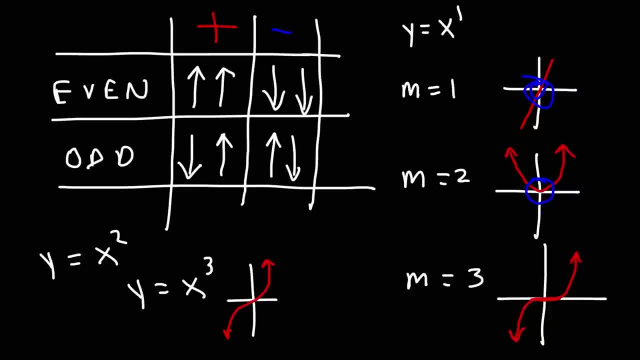 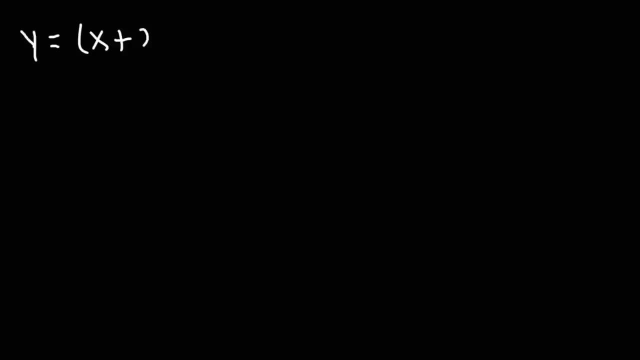 it's going to cross the x-axis, but not in a straight line, but rather with a horizontal tangent. So now let's work on some example problems. Consider the polynomial function: y is equal to x plus 2 times x minus 1 squared. 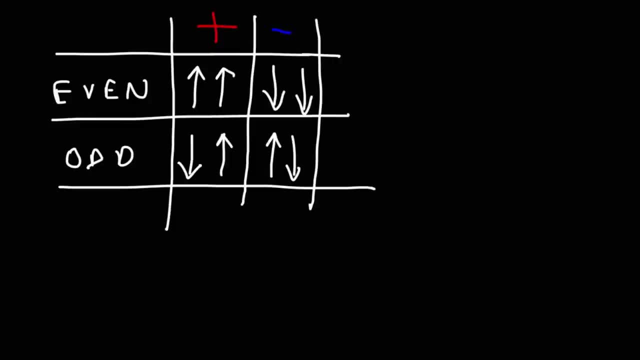 Now let's talk about the behavior of the graph near an x-intercept. I'm going to explain this more later in this video, But for now let's get started. You want to write this down. So let's say, the multiplicity of a particular x-intercept or a particular 0, is 1.. 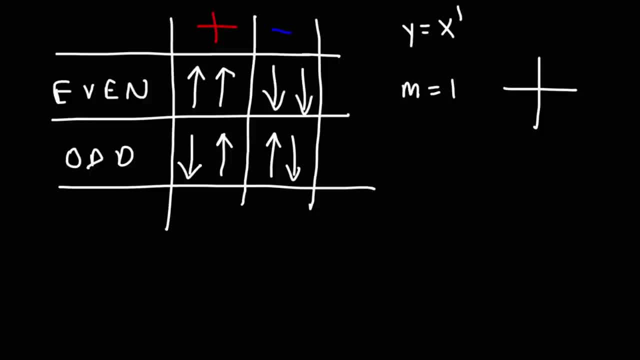 This is going to look like the graph: y equals x to the first power, So at that 0, it's simply just going to cross the x-axis, basically in a straight line. Now the angle of the straight line can vary, so you don't have to be too specific about. 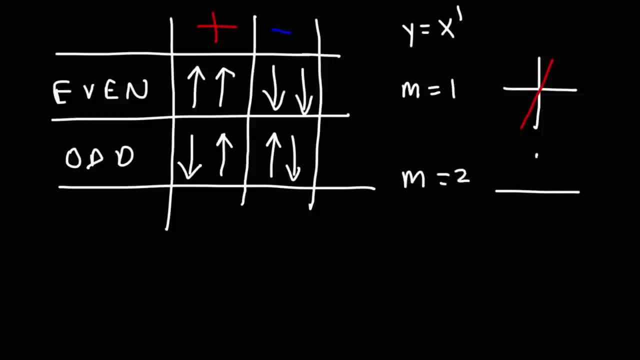 that If the multiplicity is 2, it's going to look like the graph y equals x-squared. It's not going to cross the x-axis but it's going to touch or bounce on the x-axis much in a similar way to the graph y equals x-squared. 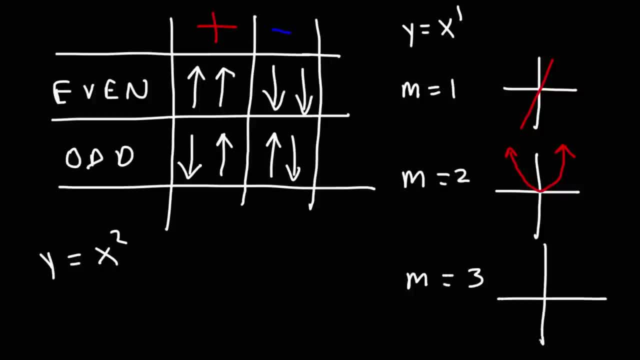 If the multiplicity is 3 for a particular 0, or x-intercept, it's going to look similar to x-cubed, but at that x-intercept. So if you think of the graph of x-cubed, it looks something like this. so you're going to have that same shape here. 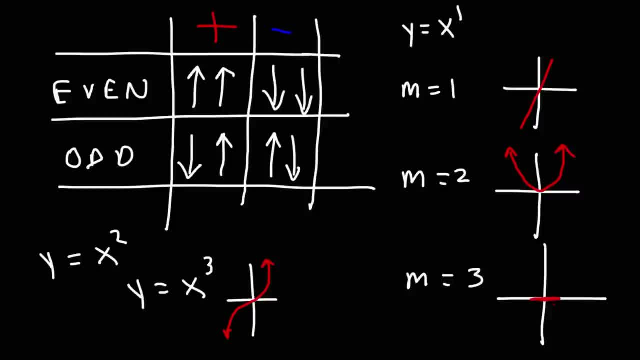 but you're going to have the behavior at that zero is going to be horizontal. so make sure you understand that if the multiplicity is one, the behavior at the x interstep is going to be like a straight line. it's going to cross the x-axis in a straight line. 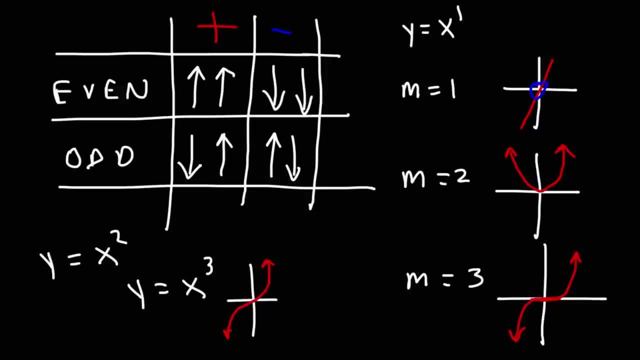 if the multiplicity is two, at that x-intercept it's not going to cross the x-axis but it's going to bounce on. you know that point. and then, if the multiplicity is three, it's going to cross the x-axis, but not in a straight line, but rather with a horizontal tangent. 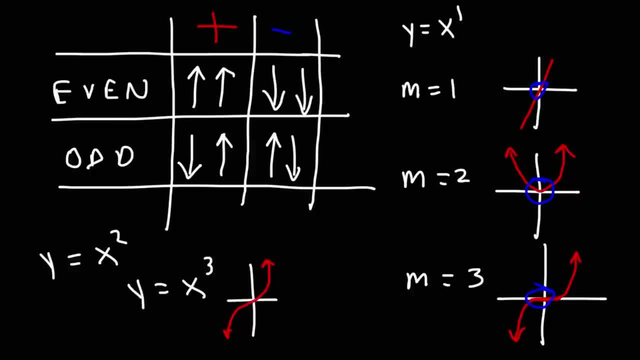 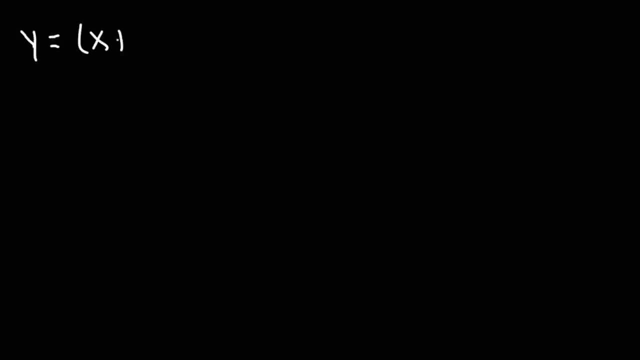 so now let's work on some example problems. consider the polynomial function: y is equal to x plus two times x minus one, squared times x minus four. so we're given a polynomial function not in standard form, but in factored form. how can we graph this particular function? 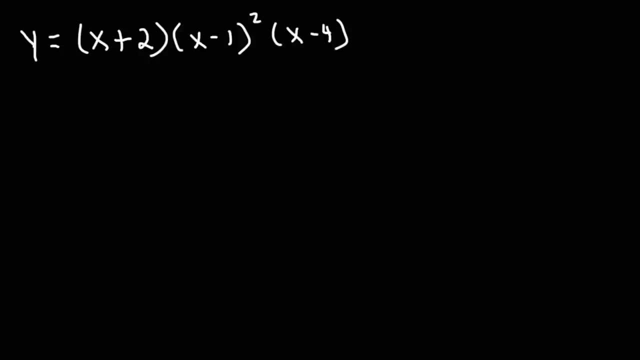 times x minus 4.. So we're given a polynomial function, not in standard form, but in factored form. How can we graph this particular function? Well, the first thing we need to do is we need to identify the zeros, That is, the x-intercepts. 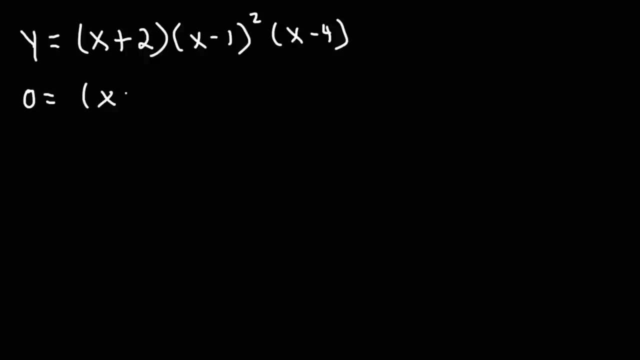 So we're going to set y equal to zero and we're going to solve for x. So in this equation, what are the possible solutions According to the zero product property? in order to solve it, we need to set each factor equal to zero. 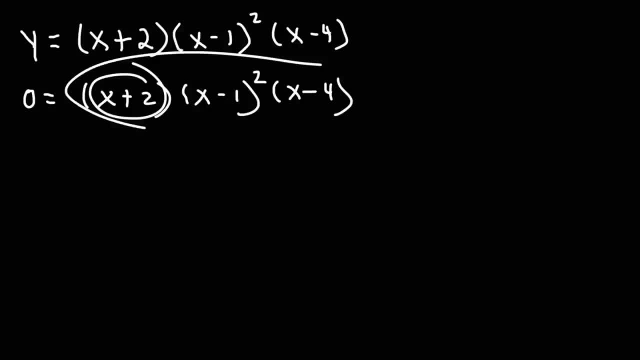 If one of these factors is zero, the entire expression on the right side will equal zero, because zero times anything is zero. So we're going to set x plus 2 equal to zero. We're going to set x minus 1 equal to zero. 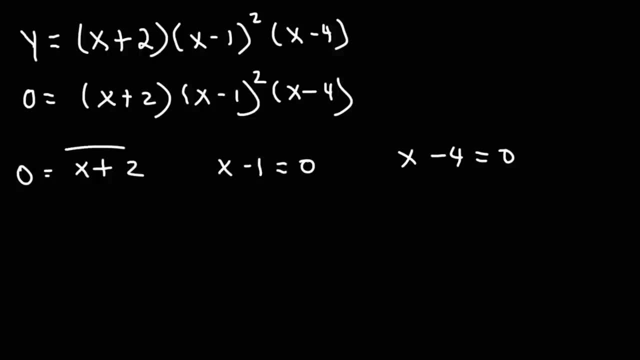 and x minus 4.. For the first equation, if we subtract 2 from both sides, we'll get that x is equal to negative. 2. For the second one, if we add 1 to both sides, we'll find that x is equal to positive 1.. 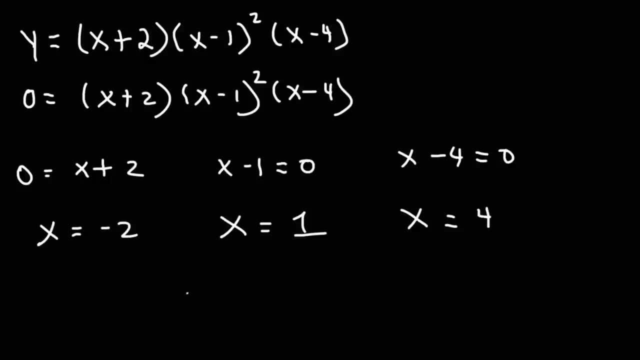 And here we just need to add 4 to both sides and then we'll get: x is equal to 4.. So that's how we could find the zeros or the x-intercepts of the polynomial function. So all we need to do 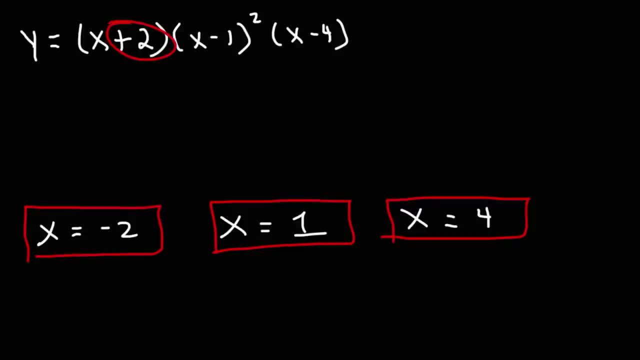 to quickly find a zero is simply replace the sign. If you see x plus 2, the zero is going to be negative. 2. If you see x minus 1, the intercept is going to be positive. 1. Here, x minus 4, just change negative 4. 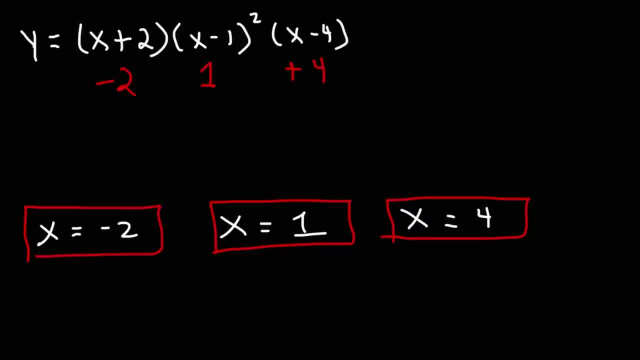 to positive 4, and that will give you the x-intercepts. Now the next thing we'll need is the multiplicity of each zero. The multiplicity is going to be equal to the exponent of each factor. So for this zero, the multiplicity is going to be: 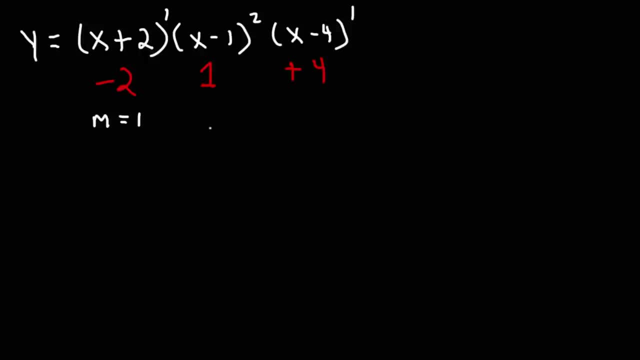 what we see here, positive 1.. For the factor x minus 1, or for the zero x equals 1,, the multiplicity is going to be 2.. And for the last one it's 1.. And so now we have everything. 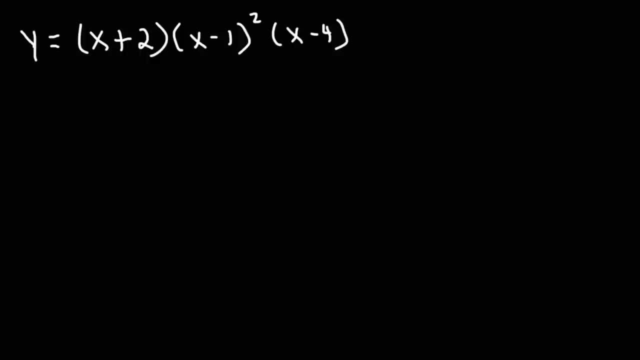 well, the first thing we need to do is we need to identify the zeros, that is, the x-intercepts. so we're going to set y equal to zero and we're going to solve for x. so in this equation, what are the possible equations for x minus two times x minus four? 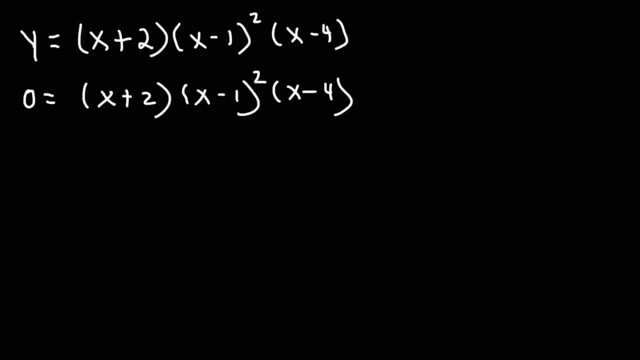 and what are the possible solutions according to the zero product property. in order to solve it, we need to set each factor equal to zero. if one of these factors is zero, the entire expression on the right side will equal zero, because zero times anything is zero. so we're going to set x plus two. 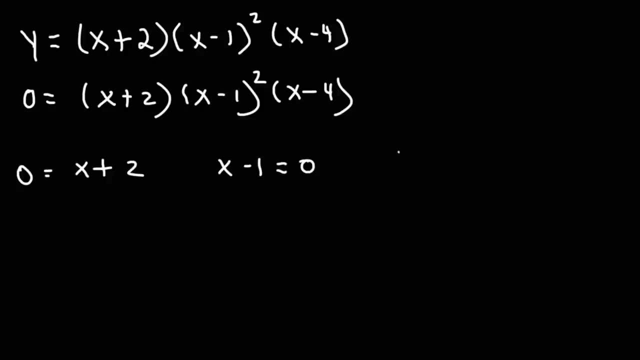 equal to zero. we're going to set x minus one equal to zero and x minus four. for the first equation, if we subtract two from both sides, we'll get that x is equal to negative two. for the second one, if we add one to both sides, we'll find that x is equal to positive one. 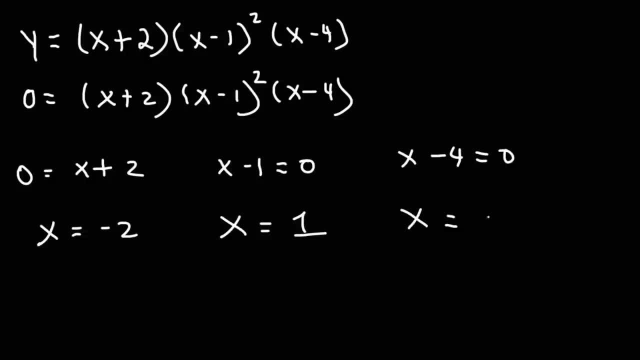 and here we just need to add four to both sides and then we'll get. x is equal to four, so that's how we could find the zeros or the x-intercepts of the polynomial function. so all we need to do to quickly find the zeros is to find the x-intercepts. 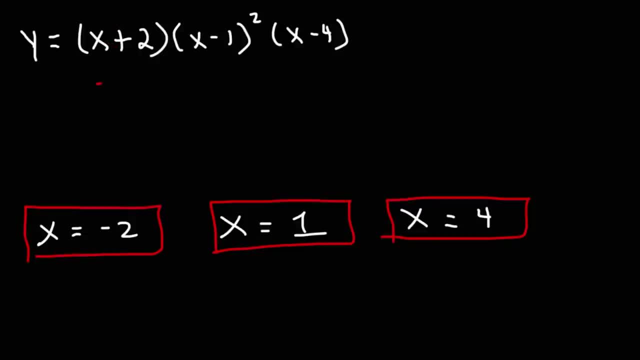 and the zeros is simply replace the sign. if you see x plus two, the zero is going to be negative two. if you see x minus one, the intercept is going to be positive one here, x minus four. just change negative four to positive four and that will give you the x-intercepts. 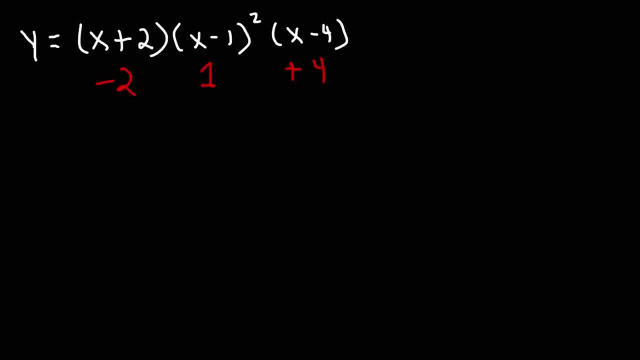 now the next thing we need is the multiplicity of each zero. the multiplicity is going to be equal to the exponent of each factor. so for this zero, the multiplicity is going to be what we see here: positive one for the factor x minus one, or for the zero x equals one. 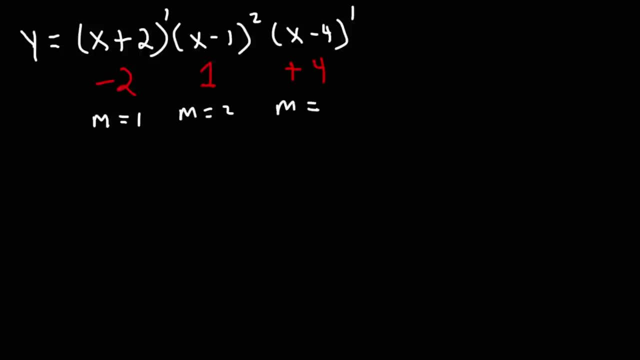 the multiplicity is going to be two, and for the last one it's one, and so now we have everything that we need in order to graph this polynomial function. so let's go four units to the left and four units to the right, so the first x-intercept on the left is at negative two. 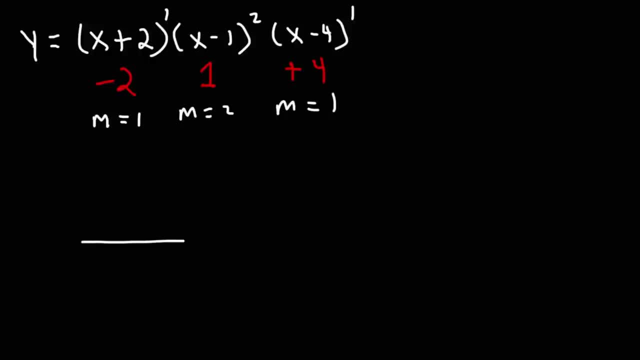 that we need in order to graph this polynomial function. So let's go 4 units to the left and 4 units to the right. So the first x-intercept on the left is at negative 2.. The second one is at positive 1.. 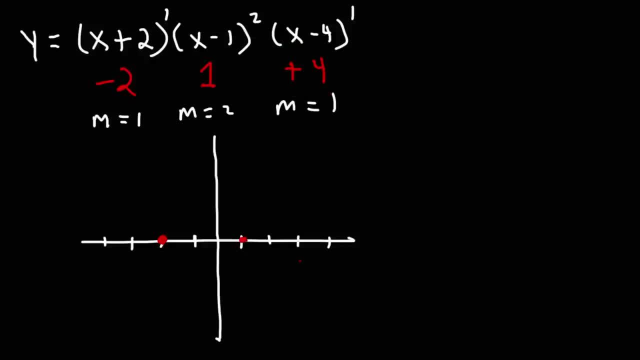 And the last one is at 4.. Now there's one more thing that we need. We need to determine the overall degree of the polynomial. To find the overall degree, simply add the exponents. 1 plus 2 plus 1 is 4.. 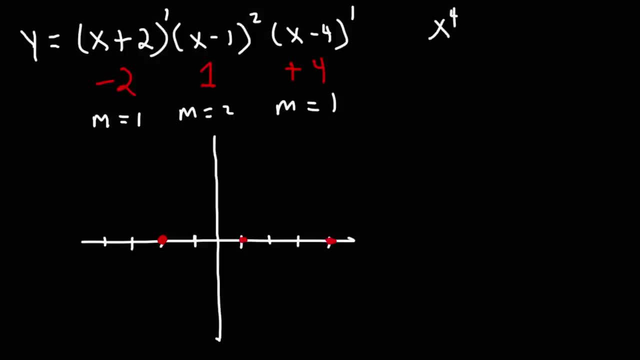 So we have a degree 4 polynomial. If you were to FOIL this entire expression, the first term will be x to the fourth, And it's positive. All of the signs here in front of x are positive. So we have a polynomial with an even. 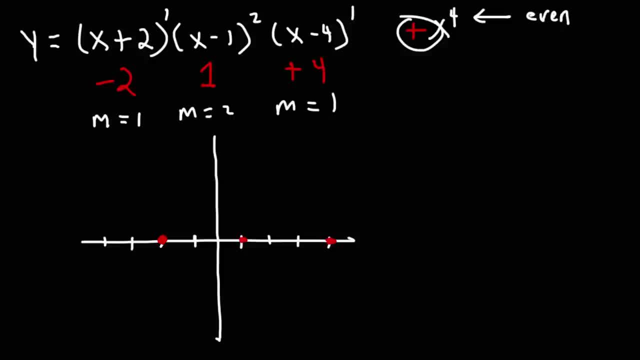 degree and a positive leading coefficient. What is the end behavior for this polynomial? If it's even, it's either up-up or down-down. Because this is positive, the end behavior will be up-up. So let's put an up arrow. 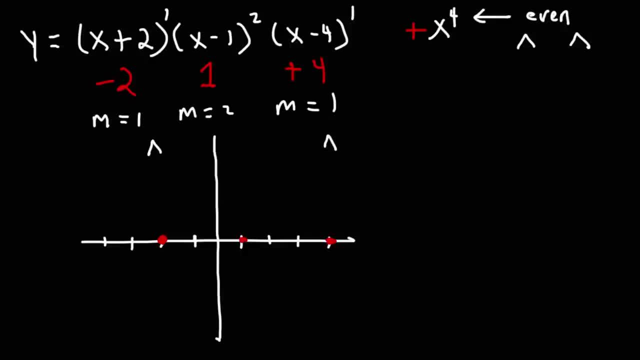 above the first x-intercept and another up arrow above the last one. So now we're going to sketch the graph from one arrow and we're going to try to connect it to the other arrow. So let's approach the first x-intercept. 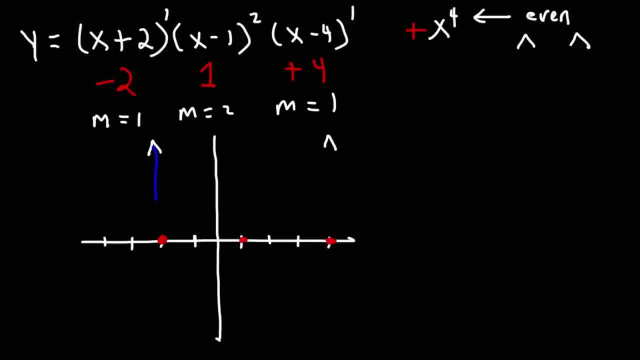 Now what is the behavior of the curve at this x-intercept? In order to find the behavior around the x-intercept, we need to look at the multiplicity. The multiplicity is 1. So the behavior is going to be similar to. 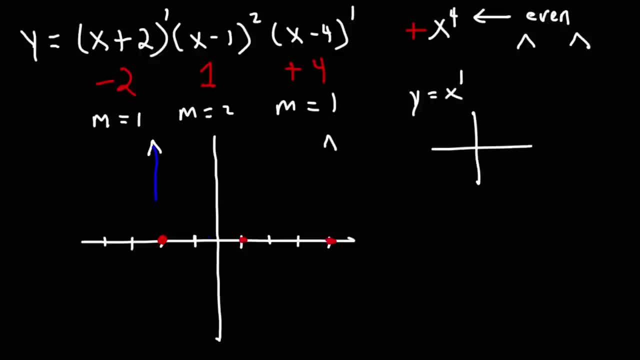 y equals x to the first power. All we're going to do is draw a straight line through that x-intercept. It's going to be linear at that point. So, because the multiplicity is 1, we're simply going to cross the x-axis. 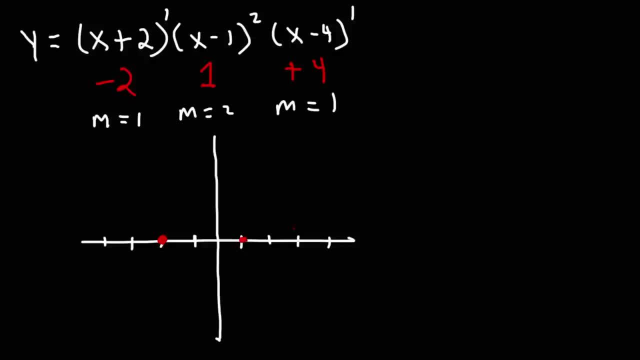 the second one is at positive one and the last one is at four. now there's one more thing that we need. we need to determine the overall degree of the polynomial. to find the overall degree, simply add the exponents one plus two plus one is four, so we have a degree four polynomial. 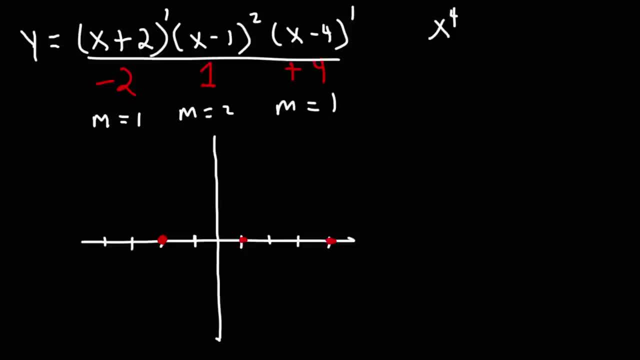 if you were to FOIL this entire expression, the first term will be x to the fourth, and it's positive. all of the signs here in front of x are positive. so we have a polynomial with an even degree and a positive leading coefficient. what is the end behavior for this polynomial? 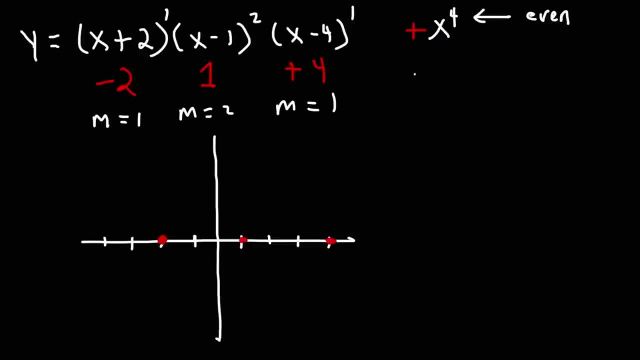 if it's even, it's either up up or down down, because the x is positive, the end behavior will be up up. so let's put an up arrow above the first x-intercept and another up arrow above the last one. so now we're going to sketch the graph from one arrow. 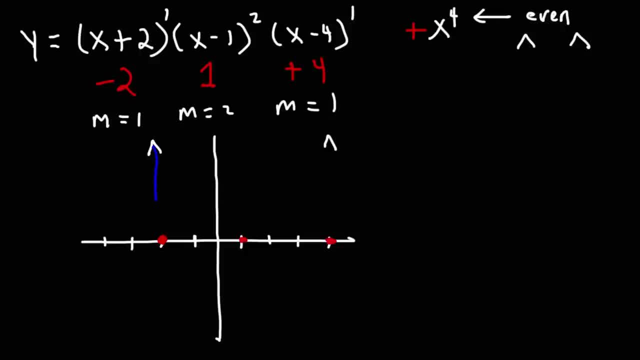 we're going to try to connect it to the other arrow. so let's approach the first x-intercept now. what is the behavior of the curve at this x-intercept? in order to find the behavior around the x-intercept, we need to look at the multiplicity. 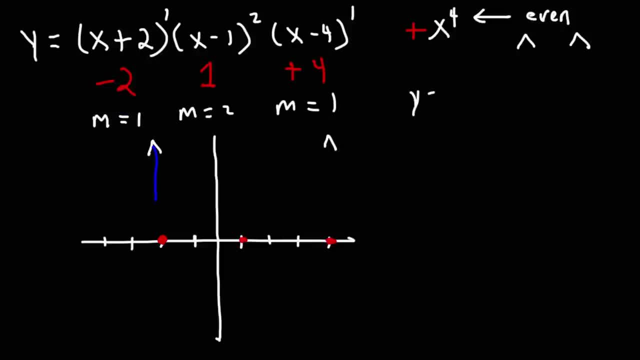 the multiplicity is one. so the behavior is going to be similar. to y equals x to the first power. all we're going to do is draw a straight line through that x-intercept. it's going to be linear at that point. so, because the multiplicity is one, 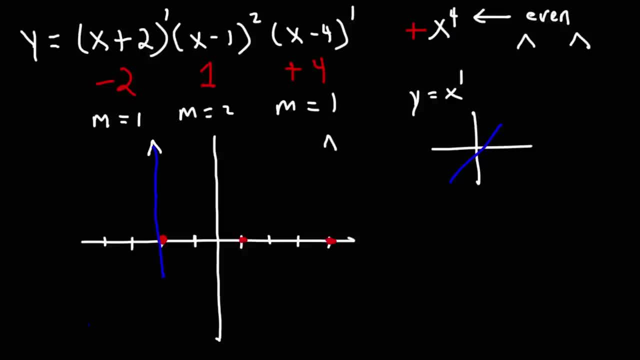 we're simply going to cross the x-axis. now we need to turn towards the next x-intercept, which is that positive one. for this one, the multiplicity is two. so think of the graph: y equals x squared. the behavior of the curve at the x-intercept. 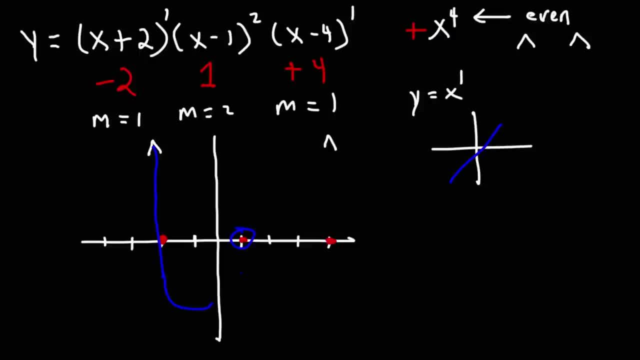 Now we need to turn towards the next x-intercept, which is that positive one. For this one, the multiplicity is 2.. So think of the graph: y equals x squared. The behavior of the curve at the x-intercept is going to look like this: 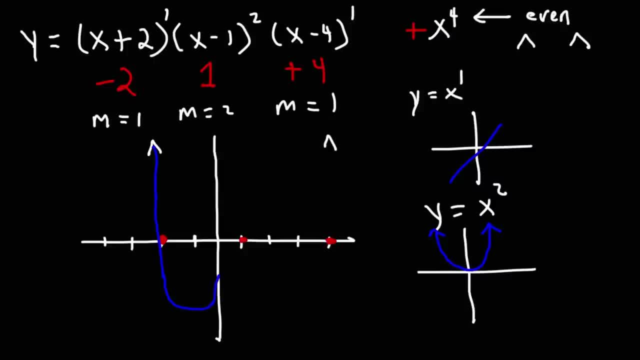 So, therefore, we're going to bounce off the x-intercept. So we're going to draw something that looks like a y equals x squared graph there, but upside down. And now for the last x-intercept. the multiplicity is 1.. 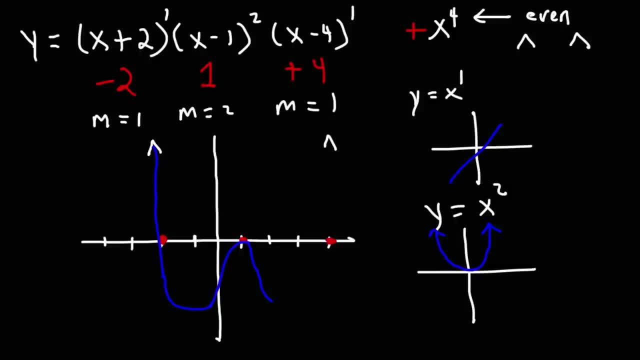 So we're going to cross the x-axis with a straight line, And so that's it. That's how we can graph this particular polynomial function. Now, the only thing we don't know is how low the peak is, or how high it is. 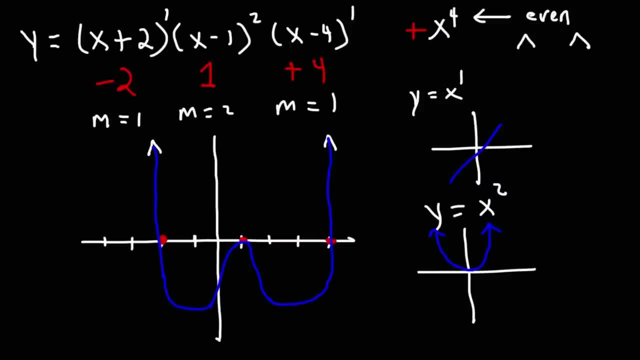 And the only way to get a good idea of the heights of those peaks is to plug in numbers. So we're going to try negative 1 and positive 2. And let's see what the y values are for those numbers. So let's plug in negative 1. 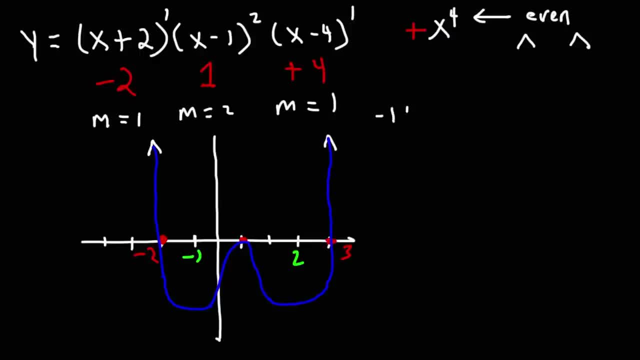 into the original expression. So we're going to have negative 1 plus 2 and then negative 1 minus 1 squared, and then negative 1 minus 4.. Negative 1 plus 2 is 1.. Negative 1 minus 1 is negative 2.. 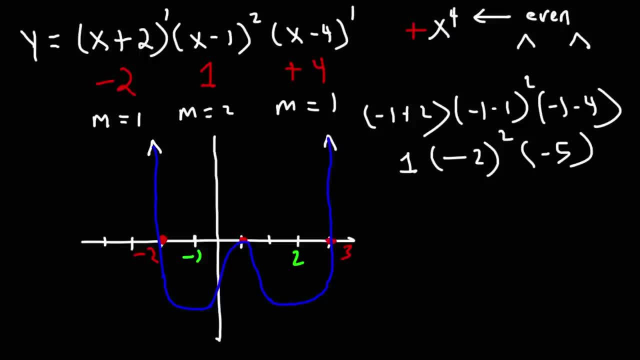 And negative: 1 minus 4 is negative 5.. Negative 2 squared is positive 4.. 4 times negative 5 is negative 20.. So that's the y value for that point. Now let's see what it is for 2.. 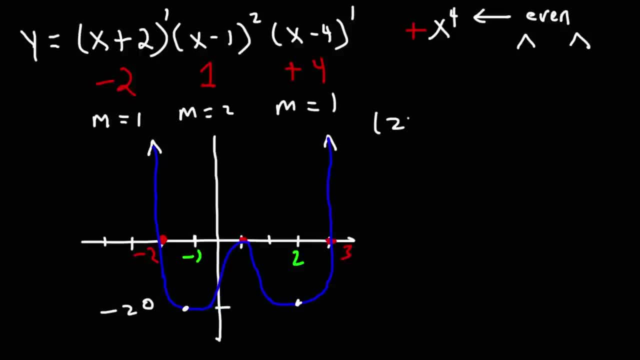 So this is going to be 2 plus 2 to the first power, 2 minus 1 to the second power, and then 2 minus 4.. 2 plus 2 is 4.. 2 minus 1 is 1. 2. 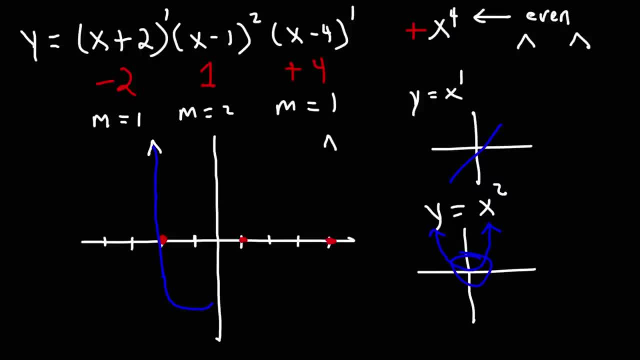 is going to look like this. so, therefore, we're going to bounce off the x-intercept, so we're going to draw something that looks like a y equals x, squared graph there, but upside down. and now for the last x-intercept: the multiplicity is one. 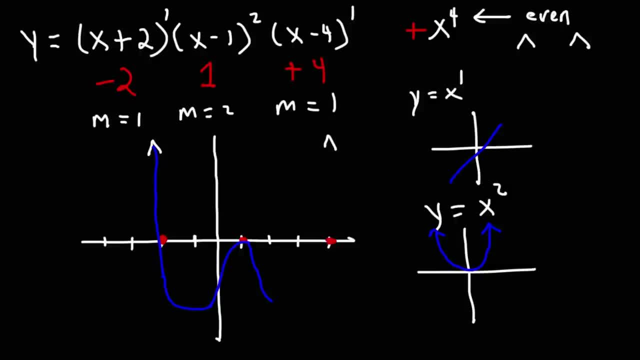 so we're going to cross the x-axis with a straight line, and so that's it. that's how we can graph for this particular polynomial function. now, the only thing we don't know is how low the peak is or how high it is, and the only way to get a good idea. 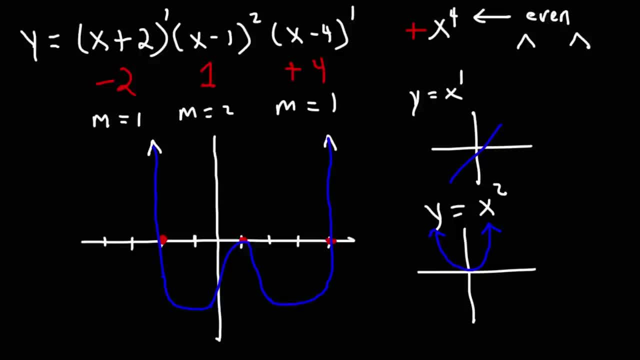 of the heights of those peaks is to draw a straight line for those peaks is to plug in numbers. so we're going to try negative one and positive two and let's see what the y values are for those numbers. so let's plug in negative one into the original expression. 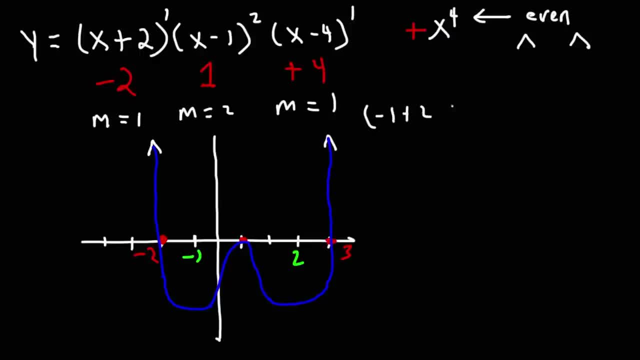 so we're going to have negative one plus two, and then negative one minus one squared, and then negative one minus one squared, and then negative one minus one, squared minus 4.. Negative 1 plus 2 is 1.. Negative 1 minus 1 is negative 2.. And negative 1 minus 4. 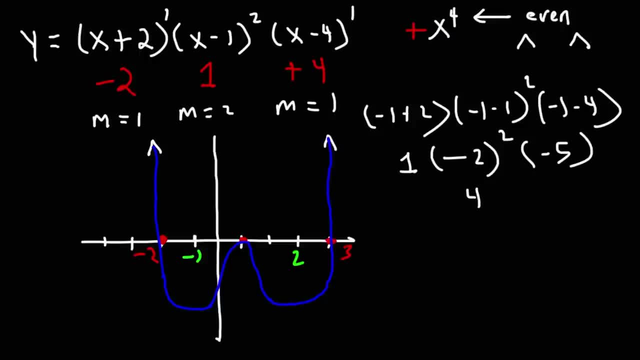 is negative 5.. Negative 2 squared is positive 4.. 4 times negative 5 is negative 20.. So that's the y value for that point. Now let's see what it is for 2.. So this is going to be 2 plus 2 to the first power, 2 minus 1 to the second power. 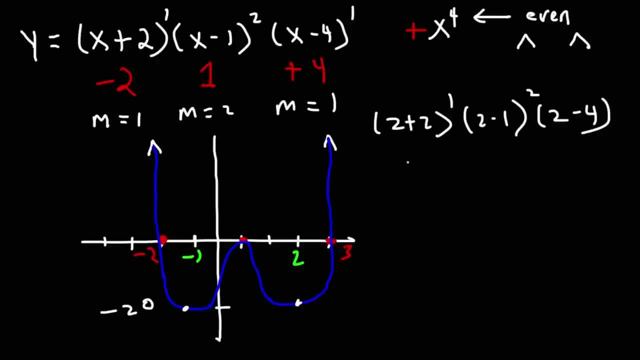 and then 2 minus 4.. 2 plus 2 is 4.. 2 minus 1 is 1. 2, I feel like I'm missing something here. 2 minus negative 4 is negative 2.. So for this one we get negative 8, which. 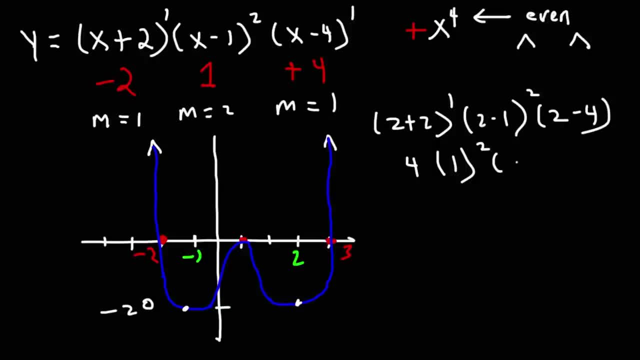 I feel like I'm missing something here. 2 minus negative 4 is negative 2.. So for this one, we get negative 8, which is not as low as negative 20.. Let's try this one. Let's try 1.. 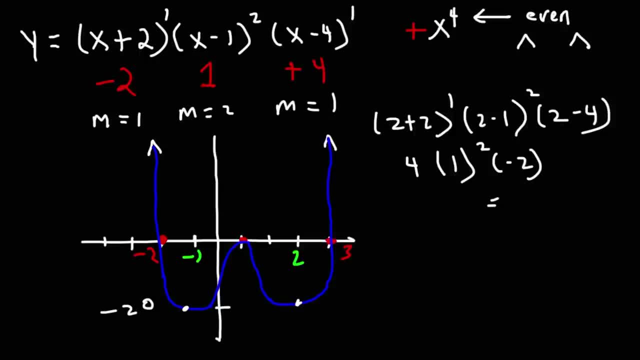 Actually, you know what? I put the wrong number. I take that back. I see the mistake I made. This is 3. And this intercept should be 4.. So this should be 3 plus 2 and then 3 minus 1 squared. 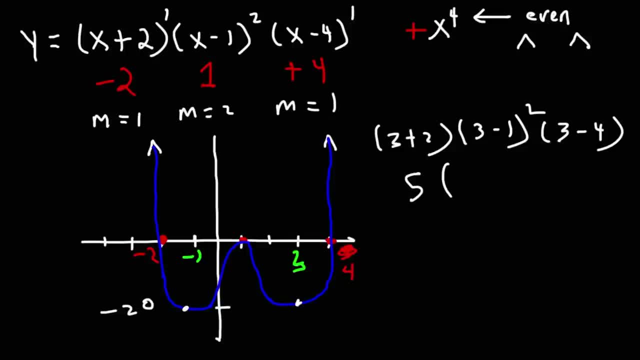 and then 3 minus 4. 3 plus 2 is 5.. 3 minus 1 is 2.. 3 minus 4 is negative 1. 2 squared times 4 times negative 1. That's negative 20.. 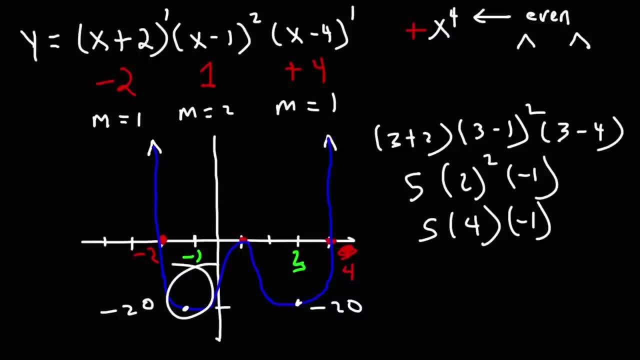 Okay, So these two peaks are of the same height for this particular example, And you can see why There's symmetry, so to speak. These two zeros have the same multiplicity And the distance between these two x-intercepts they're the same. 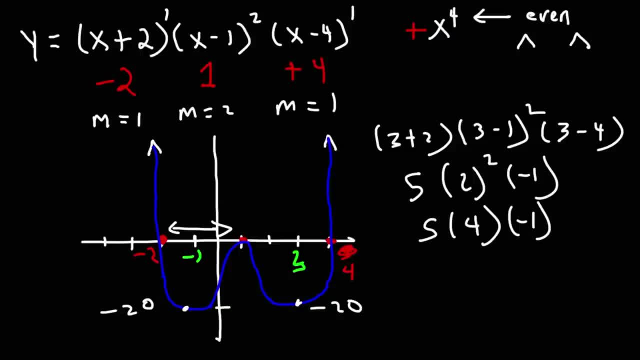 So, due to the fact that this graph is symmetric, about x equals 1, we can see why these two values are the same. Now, this is not going to be the case for every other example, It's just for this particular example. So the best way to determine 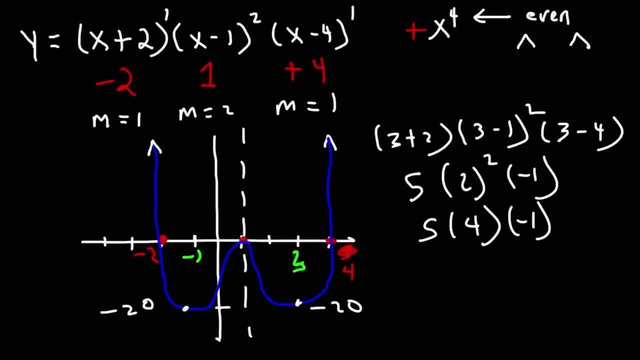 the relative heights of the peaks is simply to plug in numbers. In this case, they just happen to be the same. 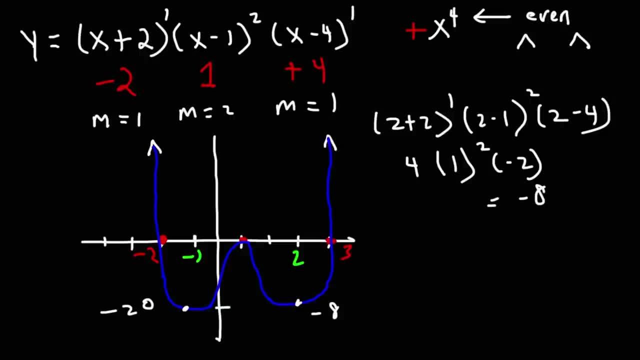 is negative 8.. It's not as low as negative 20.. Let's try this one. Let's try 1.. Actually, you know what? I put the wrong number. I take that back. I see the mistake I made. This is 3, and this intercept should be 4.. 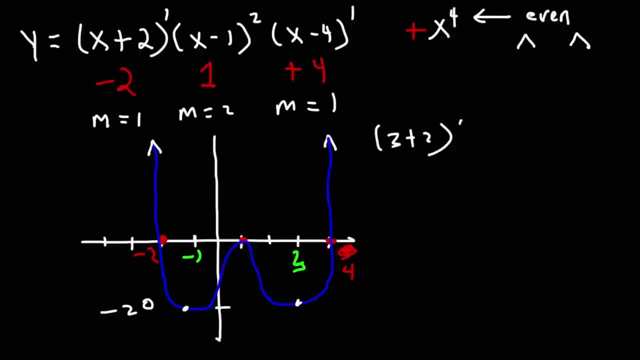 So this should be 3 plus 2, and then 3 minus 1 squared, and then 3 minus 4.. 3 plus 2 is 5.. 3 minus 1 is 2.. 3 minus 4 is negative. 1. 2 squared times 4 times. 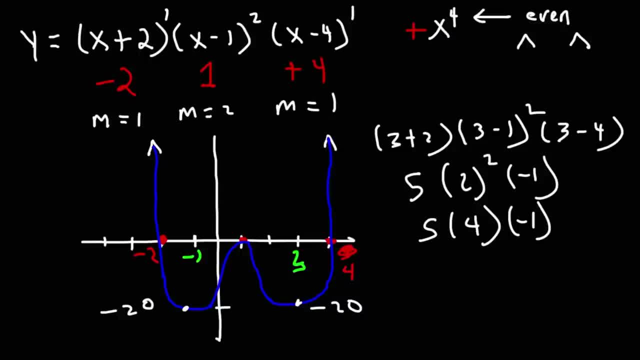 negative 1, that's negative 20.. Okay, so these two peaks are of the same height for this particular example, And you can see why There's symmetry, so to speak. These two peaks are of the same height for this particular example, And you can see why There's symmetry, so to speak. 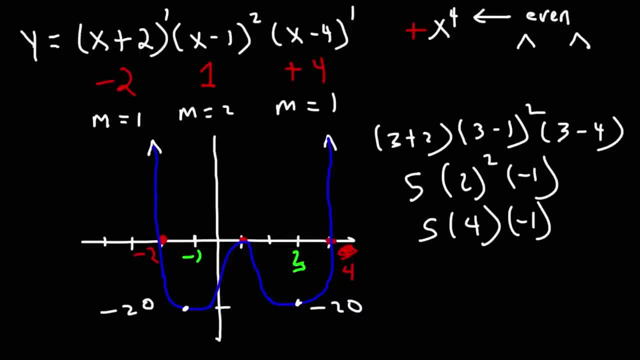 These two zeros have the same multiplicity and the distance between these two x-intercepts they're the same. So, due to the fact that this graph is symmetric, about x equals 1, we can see why these two values are the same. Now, this is not going to be the case, for 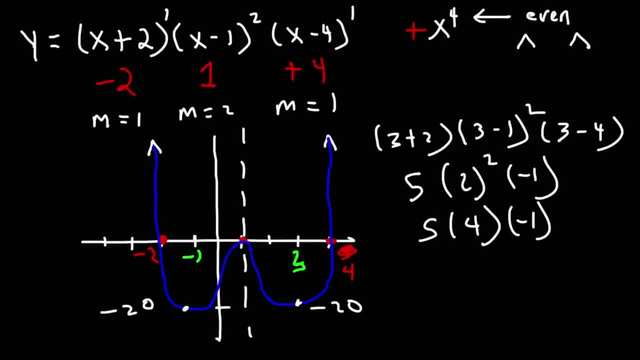 every other example, It's just for this particular example. So the best way to determine the relative heights of the peaks is simply to plug in numbers. In this case they just happen to be the same. 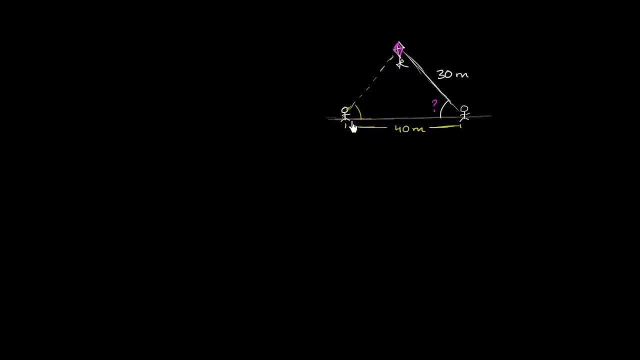 Say, you're out flying kites with a friend and right at this moment you're 40 meters away from your friend and you know that the length of the kite's string is 30 meters and you measure the angle between the kite. 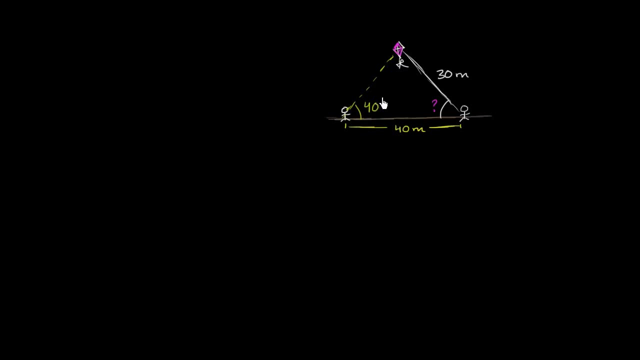 and the ground where you're standing, and you see that it's a 40 degree angle. And what you're curious about is whether you can use your powers of trigonometry to figure out the angle between the string and the ground. And I encourage you to pause the video now.